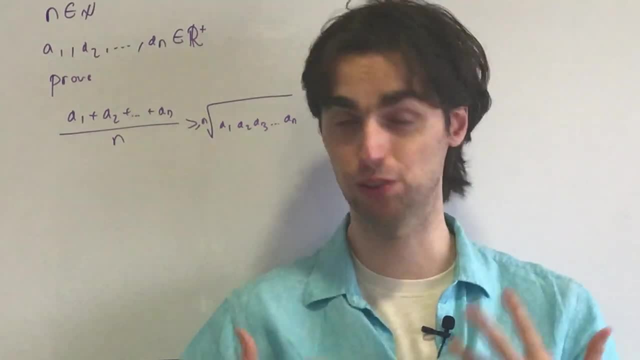 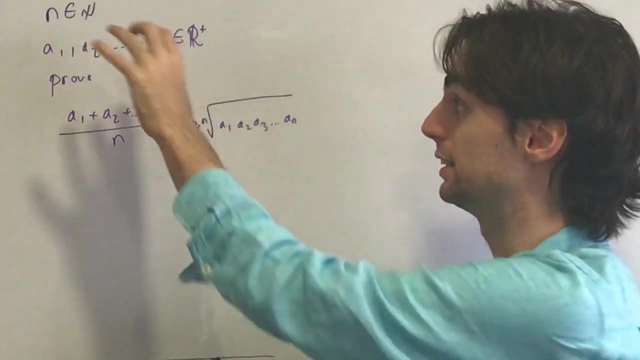 let's think about it. what is this one problem-solving principle we talked about here? well, we say that, listen, if you want to prove something general, try to prove it for specific, small cases. this is a general and a general a 1 through a n. let's try to prove it for one specific a. 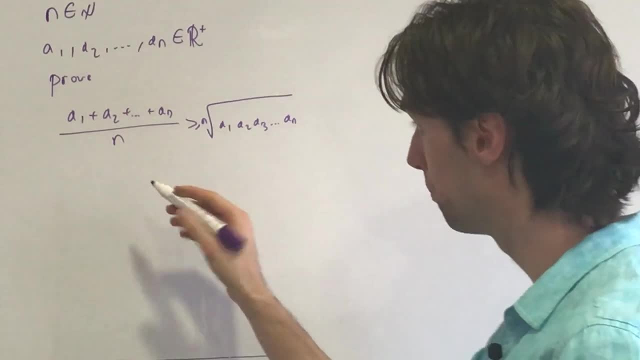 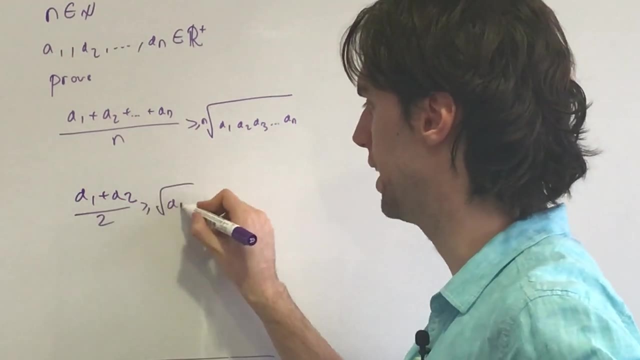 1, namely- let's try to prove it- for n equals 2, for n equals 2, we have this is a 1 plus a 2 over 2 is greater or equal to the square root of a 1 a 2, and we know. 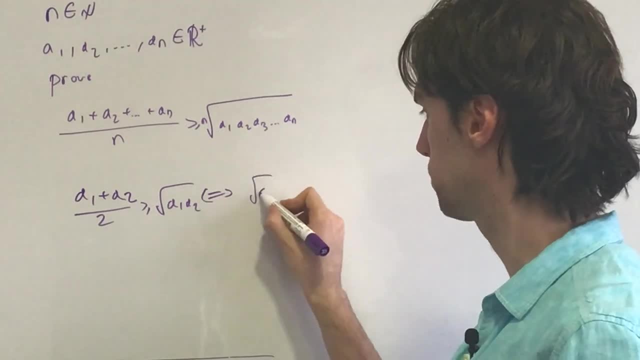 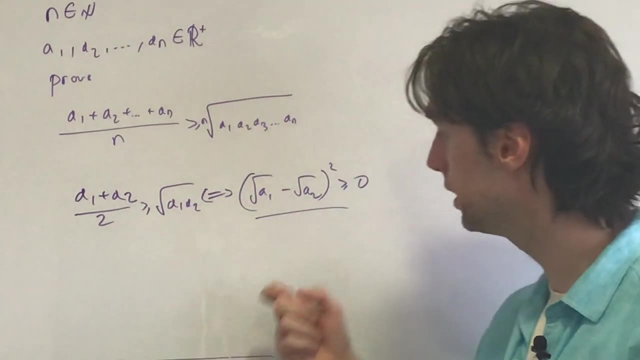 that we can write this down. this is true if, and only if, the square root of a 1 minus square root of a 2 squared is greater or equal 0, which is true. we have equality if, and only if, these two numbers inside a square roots are equal. 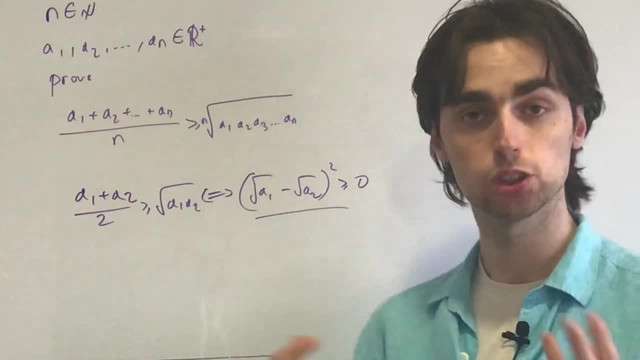 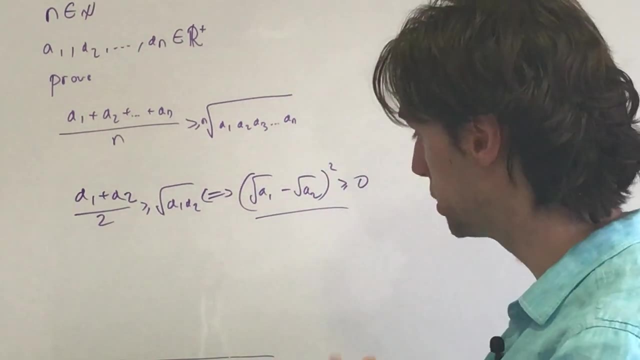 and they are equal only if it 1 and 2. if a1 and a2 are equal. So we have this sort of basic thing proved. Now can we prove a3? Well, for a3, we have a bit of a difficulty. 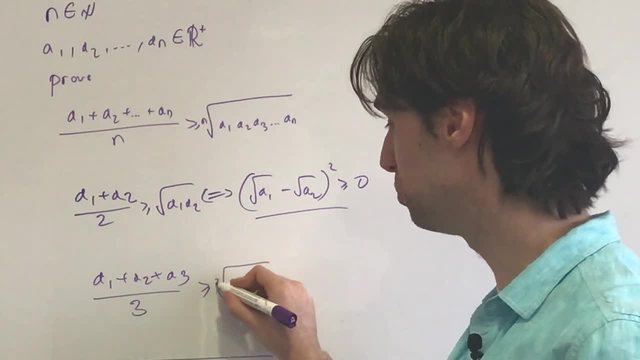 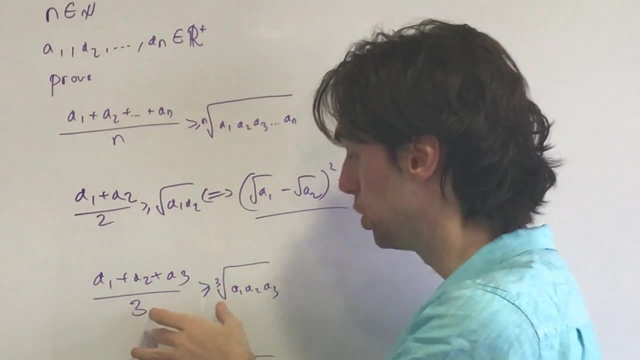 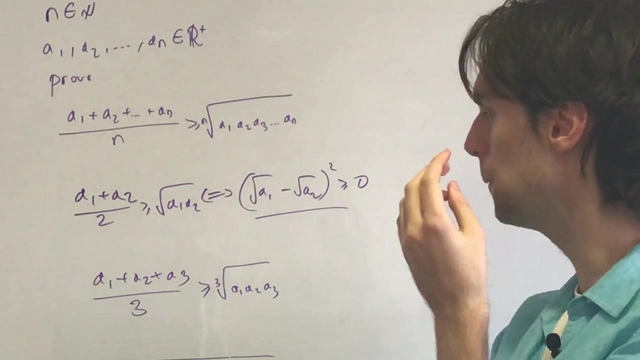 Like right, this is over 3 greater than or equal to the cube roots of a1, a2, a3.. Now, if we were to cube everything, we could do this. We could prove this potentially, maybe- Actually, I'm not even sure- 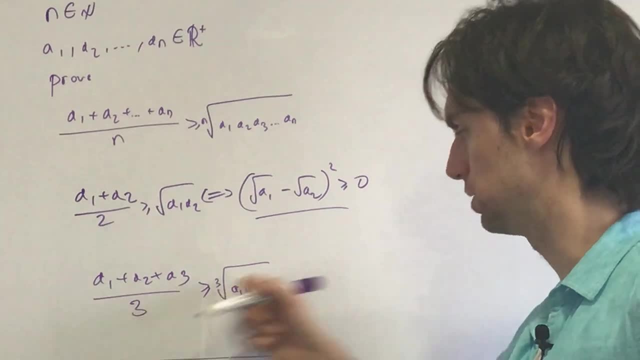 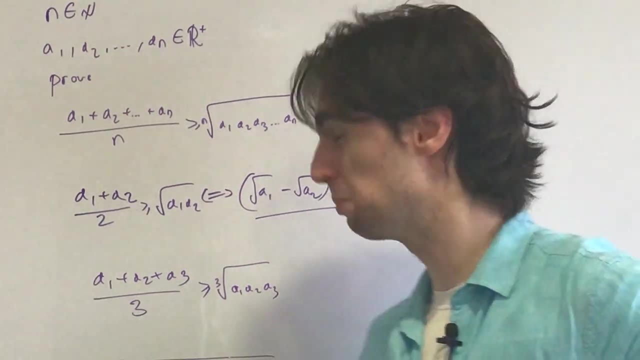 What would we have If we cubed this, multiplied this by 27, and cubed it? we would have a1 to the power of three b, a2 to the power of three, a3 cubed, and then all those combinations of them. 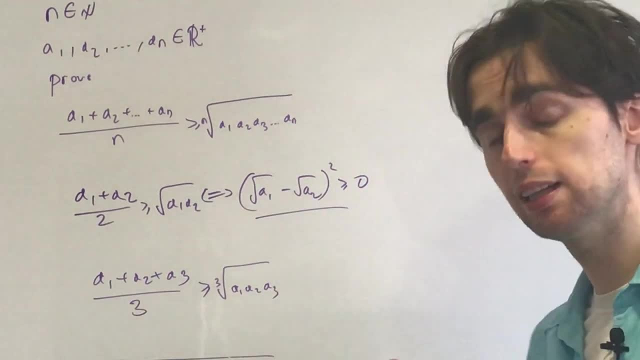 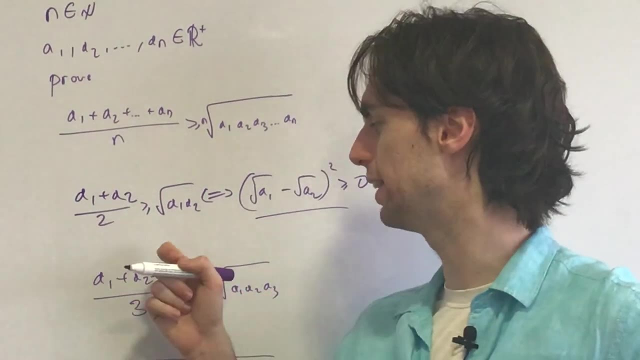 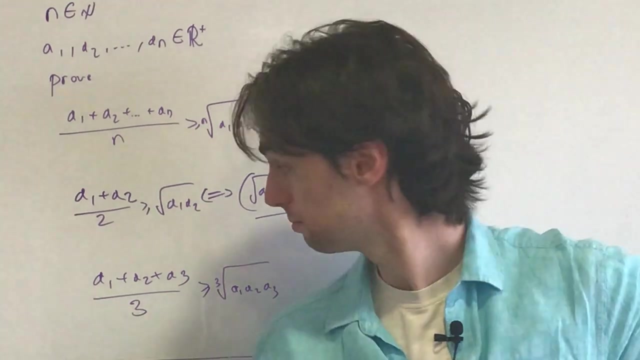 Now we could, and we would end up. we would still end up needing to prove that a1 cubed plus b1 cubed plus a1 cubed plus a2 cubed plus a3 cubed is greater than or equal to three: a1, b1, c, a1, a2, and a3. 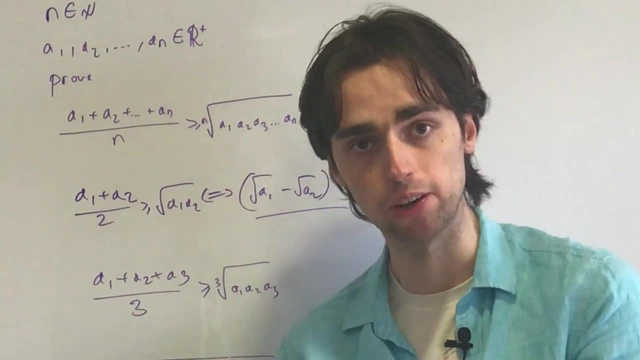 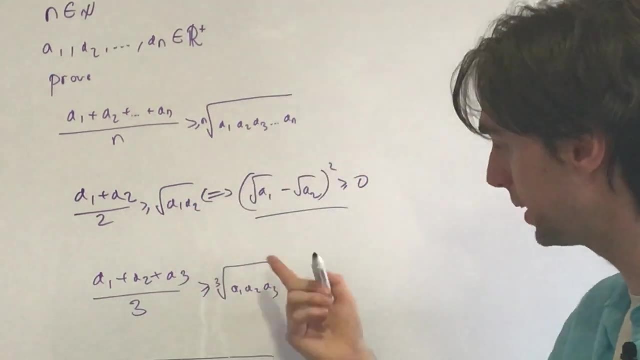 And we would still have to prove like really the same thing here. It's just like with a different name. So cubing, it doesn't really solve anything. It just- I mean it gets rid of the root. but we can get rid of this root by saying: let ai be equal. 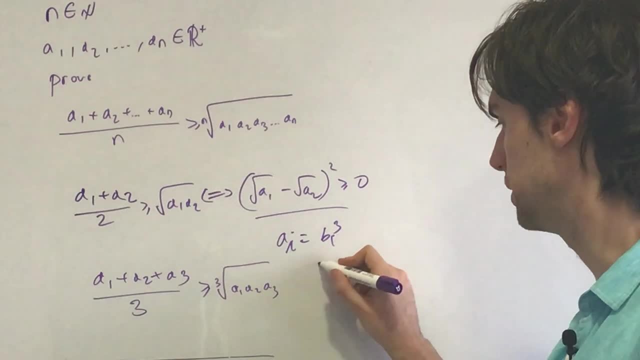 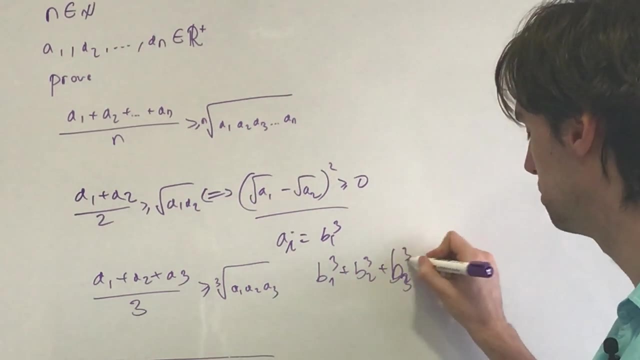 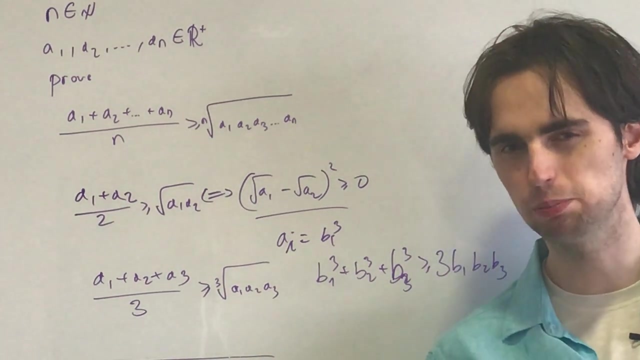 equal to bi cubed. and then what we need to prove is that b1 cubed plus b2 cubed plus c2 plus b3 cubed is greater than or equal to three: b1, b2, b3.. And now there doesn't seem to be a very 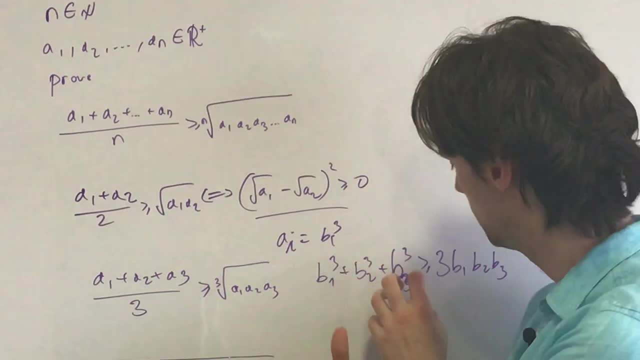 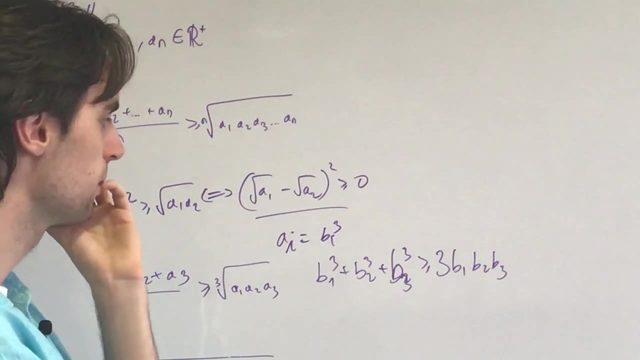 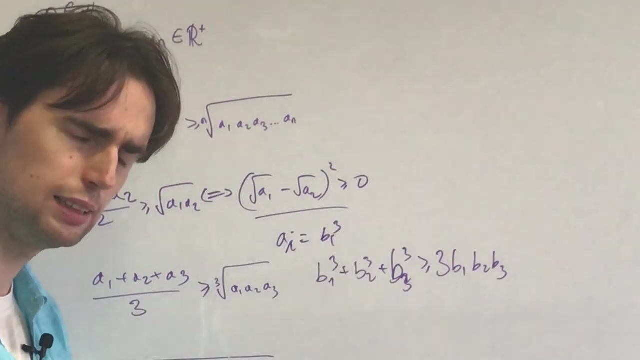 how should I say this? A very direct, a very intuitive way as to how we should actually go about factoring this right. So okay, three seems to be difficult. Now let's do a thing where we let's forget about three for a bit. 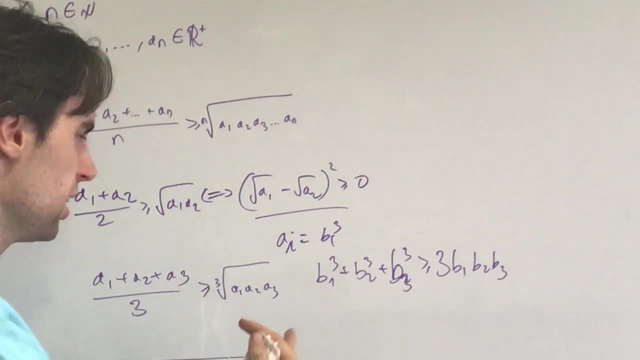 Let's look at four, because we're having maybe trouble here, Maybe there's other cases we can solve and maybe we can use something there to solve these smaller cases. And this is a bigger, a more higher order problem-solving strategy is. 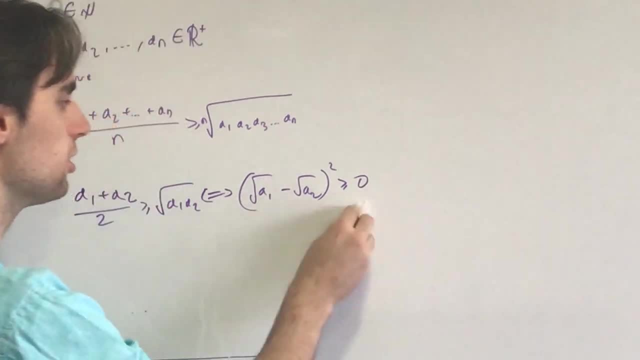 when you can't figure something out, try to see if there's something else you might figure out on another case that could be useful. on a lower case Now, for n equals four, what do we have? We need to prove that. let's just use a plus b. 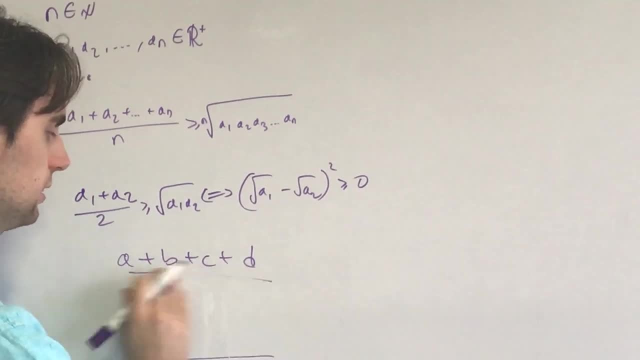 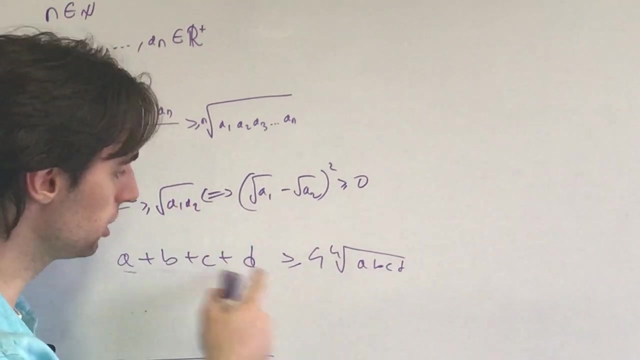 plus c plus d over four. actually, this is greater or equal to four times the fourth root of a, b, c, d. right Now, can we prove this in any way, shape or form? And the answer here is: I invite you to actually hear. 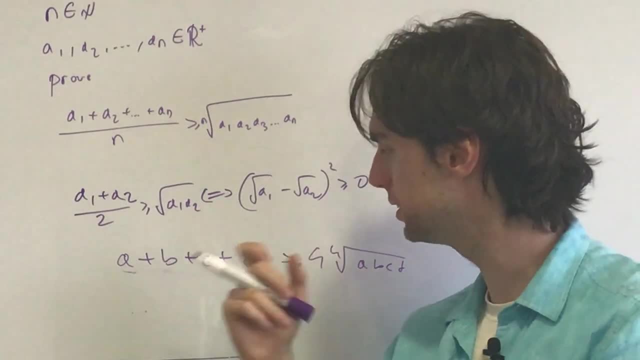 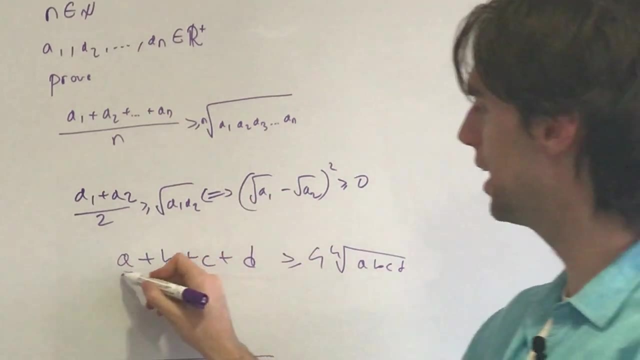 pause for, say, five minutes and see if you can prove this fact. okay, Now I hope you've paused. Well, look, if we apply this thing up here on a plus b, this is going, this thing, right. 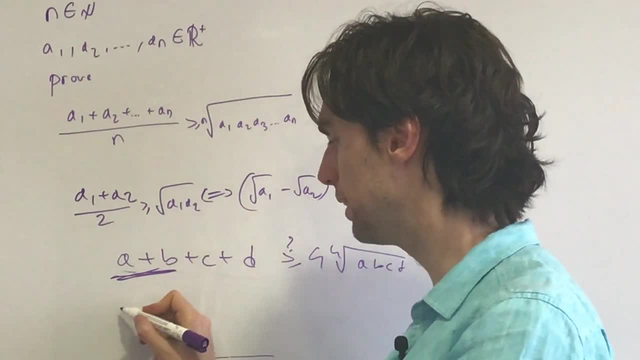 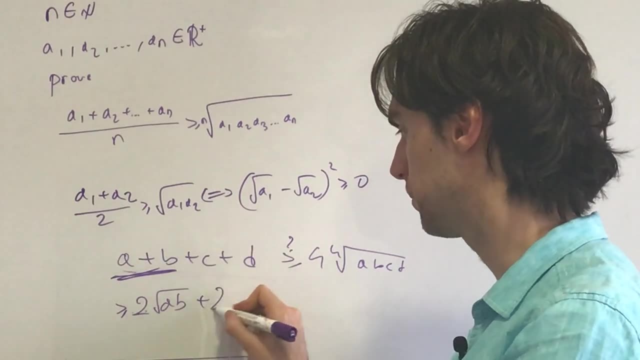 this is a question mark, right? We don't know if this is true, But we know that a plus b is greater or equal to two roots of a- b, and this thing right here is greater or equal to two square roots of c- d. 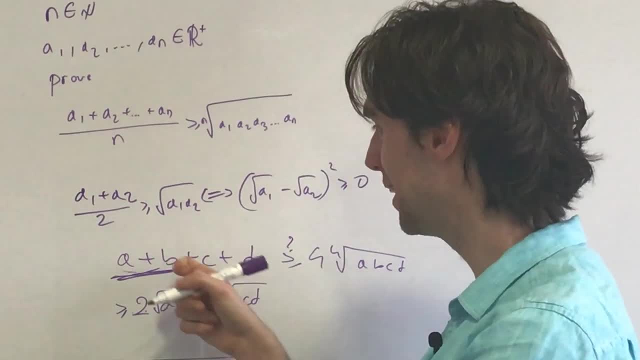 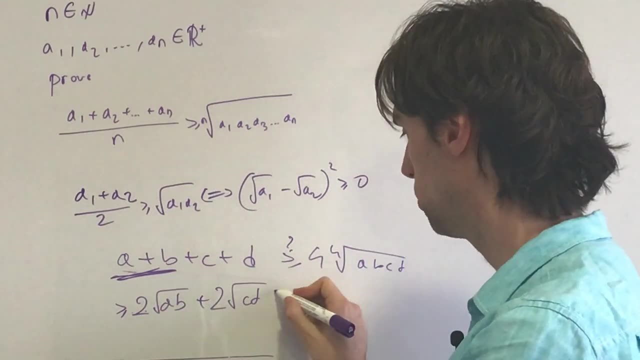 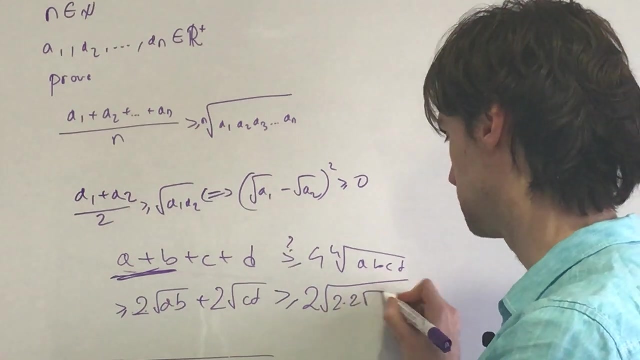 Right. And now, if we apply the same thing again on the square root of a, b plus- we can do two times this- we'll have that this is greater or equal to two times the square root of two times two times square root of a, b times square root of c, d. 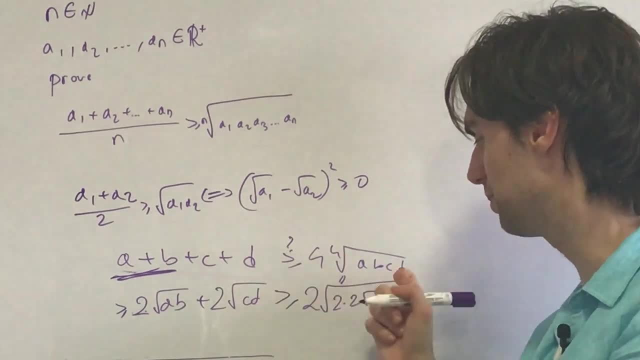 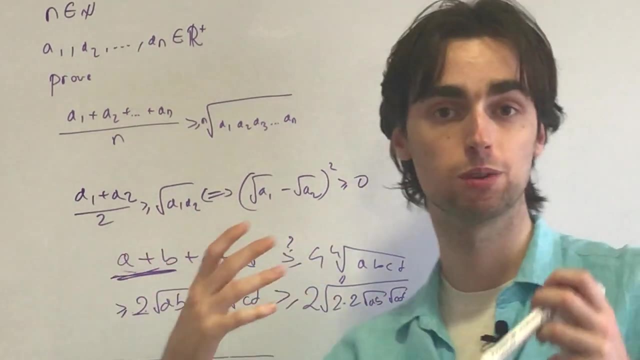 which is equal to this four times the fourth roots of a, b, c, d, right. So for n equals four. we can actually solve this And if you think about it well, we can also solve for n equals eight right. 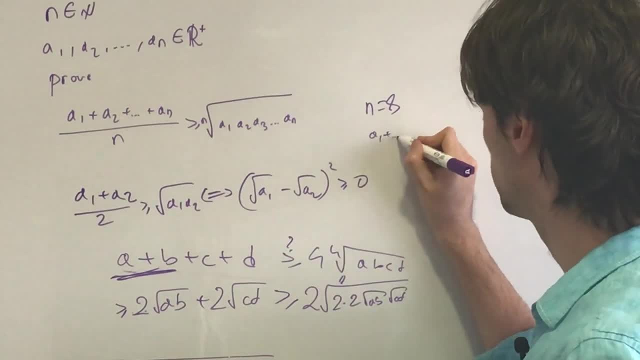 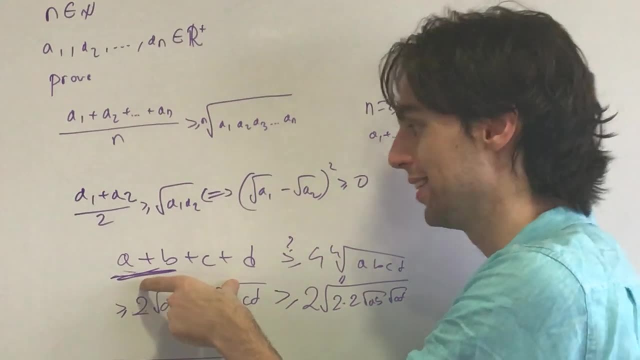 It's just going to be, we'll apply. so we have a one plus all the way to a eight. We'll know this is greater or equal to. well, by this thing right here, we'll know this is greater or equal to. 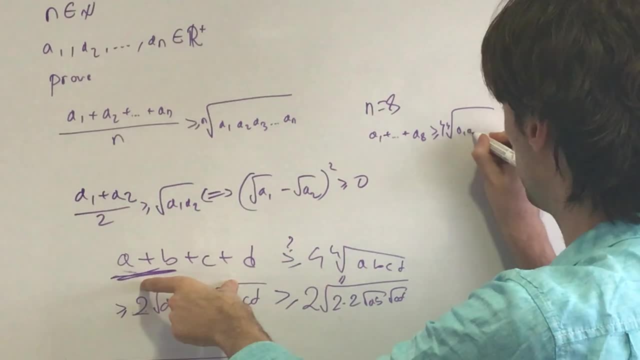 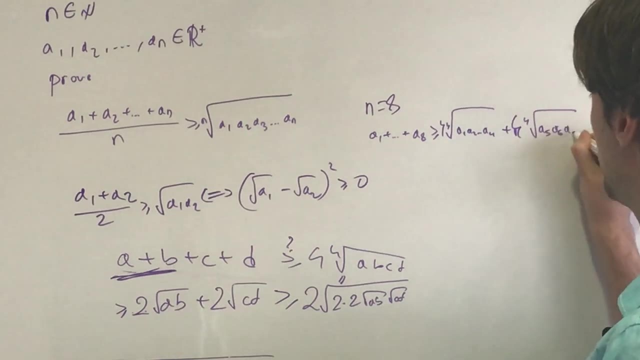 the fourth times the fourth roots of a, one a two to a four, plus four times the fourth root of a, five, b, c, d. So that's going to be a one plus all of this, plus five a, six, a seven. 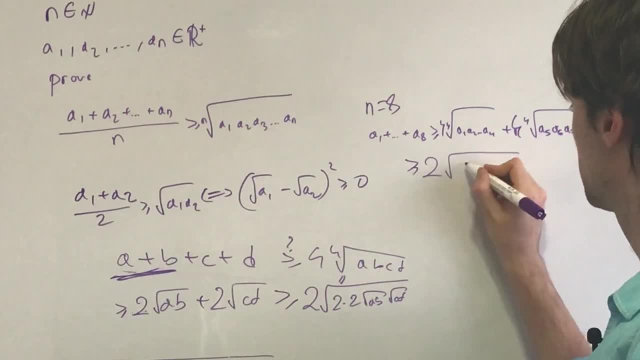 a eight. and then, when we apply this thing right here, this will be greater or equal to two times square roots of four times four, the eighth root of a one. a eight, the fourth root of this. And when you get rid of the square root, 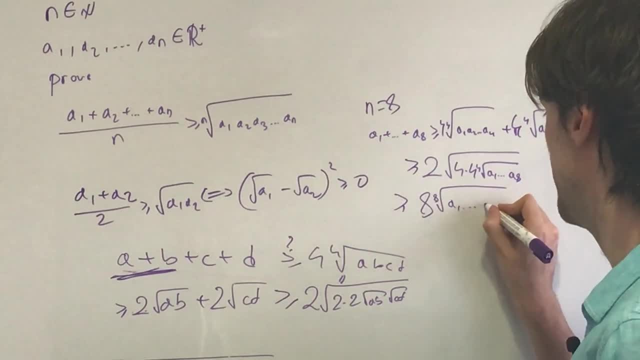 you have eight square eight roots of a, one through a, eight right. So now what we have is: we have anywayspace ancientTEXualôn greater or equal to b, one b Y equals 1.. you have eight square eight roots of a, one through A, eight. 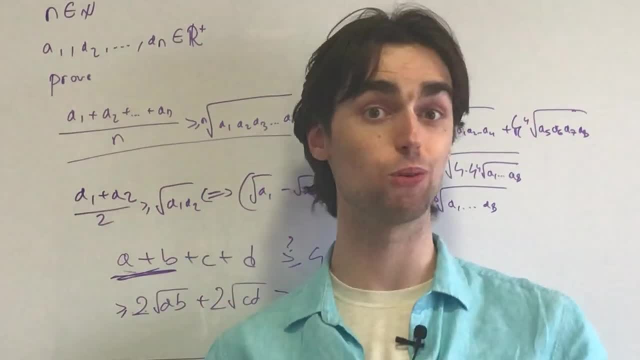 right, I'm just gonna stop there. so now what we have is: we have adios, all right, a quarter two, five, a number two, n, seven, t, ten. this inequality proved for every power of two. now my question for you is: can we use the fact that? 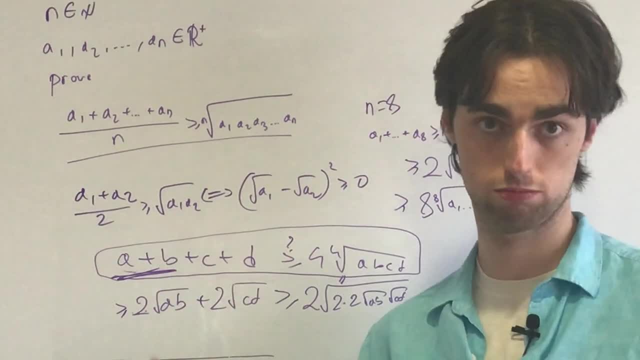 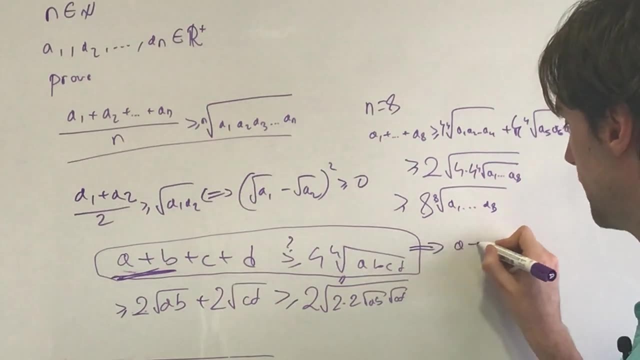 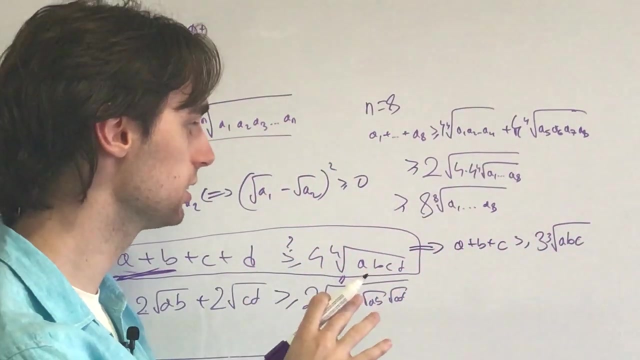 this is always true. somehow can we use the fact that this is always true to prove that from here that it follows that a plus b plus c is greater than or equal to three cube roots of abc. can you use this to prove this? i invite you here to pause, for about say: 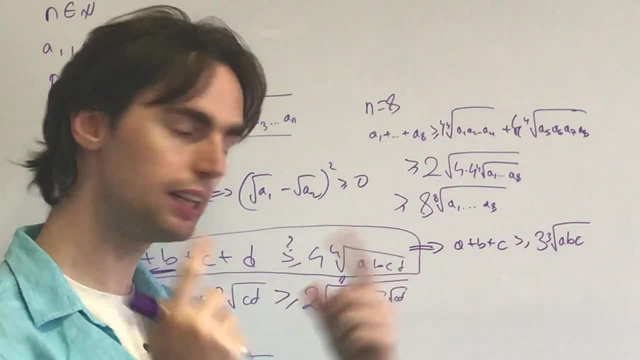 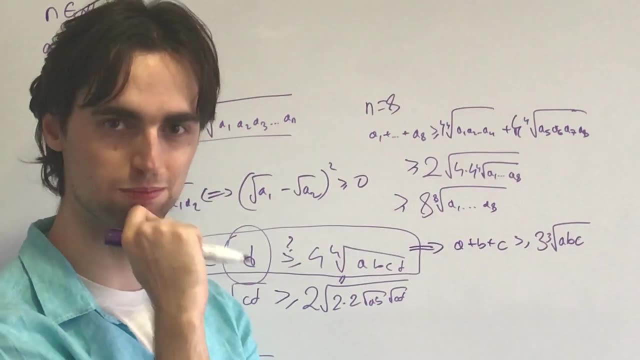 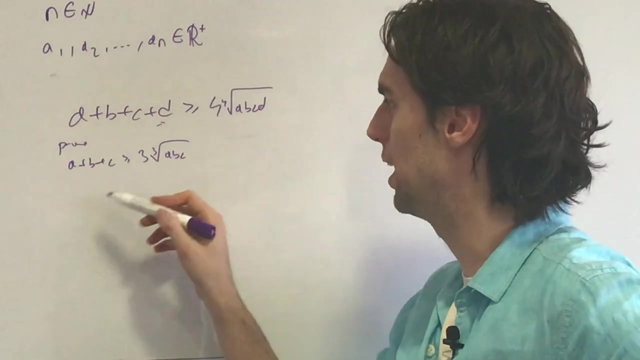 take 15 minutes and try to think about: can you set d to something so that this thing here implies this pause now, and here's the next step, okay, so now we need, so we need to set d somehow such that this thing becomes zero, this thing right, when we move d to the other side, that it becomes this: 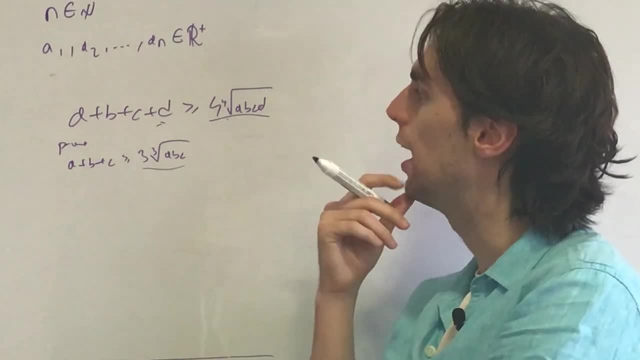 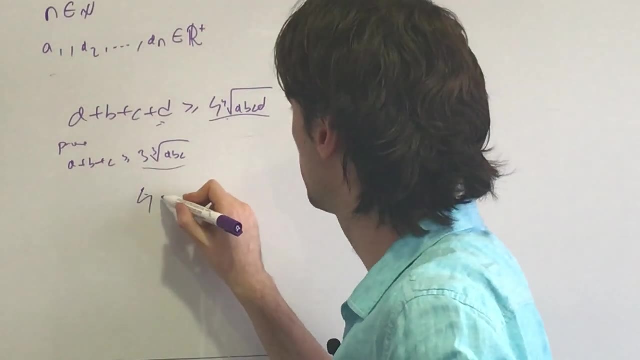 so let's actually set that up as some sort of like equation. uh, i mean, that's one thing we could do. we could just like set this up as an equation. we need to have what we need. we need four times the fourth root of abcd minus d to be equal to three times. 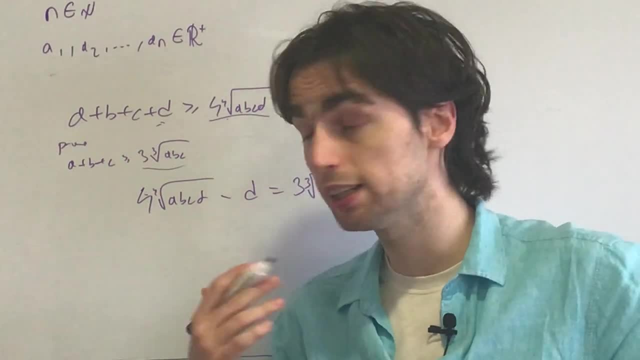 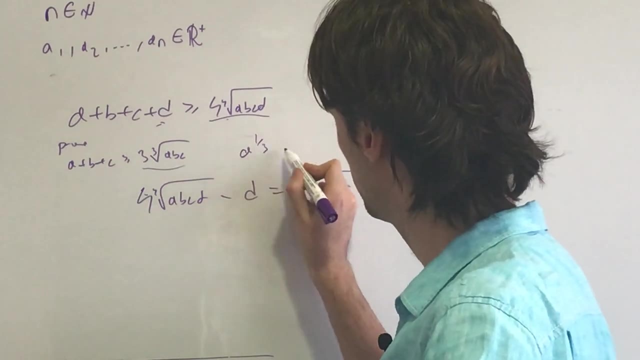 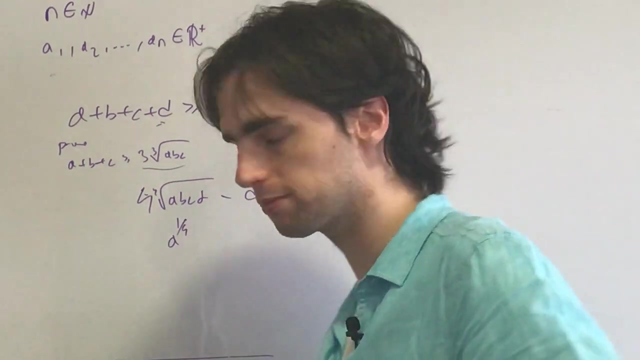 the cube root of abc, right. that's one way of thinking about this. another way is say: okay, this is all. this thing is a to a third, b to a third, c to a third. here we have a to a fourth right. i need to make a to a fourth when i'm multiplied by d to be a to a third right. 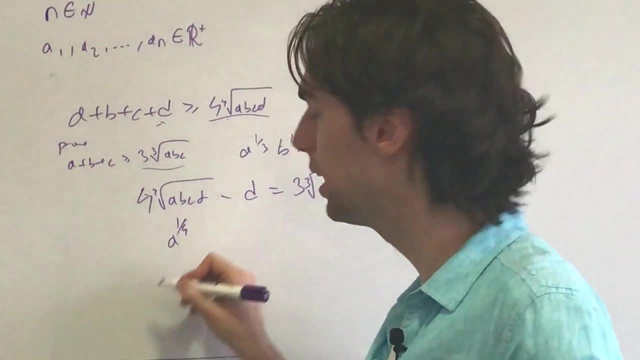 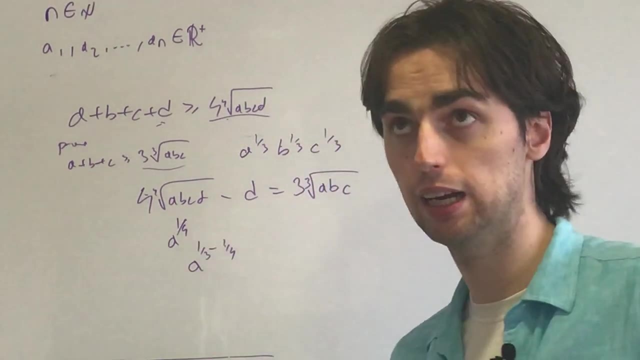 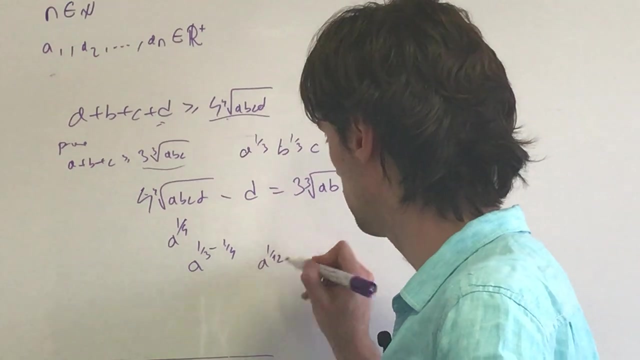 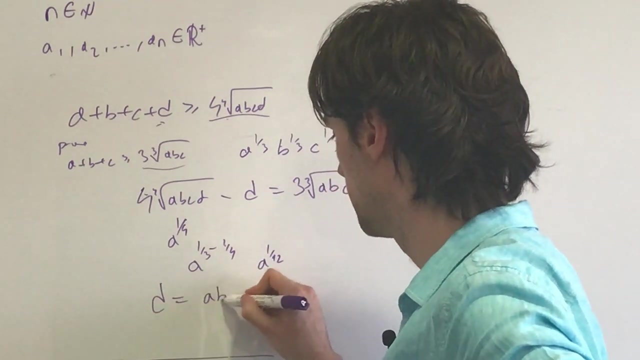 so i need in d, i need to have what i need to have it a to d, one third minus a fourth. now, what is that? well, that is four, three. that is a to one over twelve, right? so what do we have when we set d to equal to abc, to the power of one over twelve? 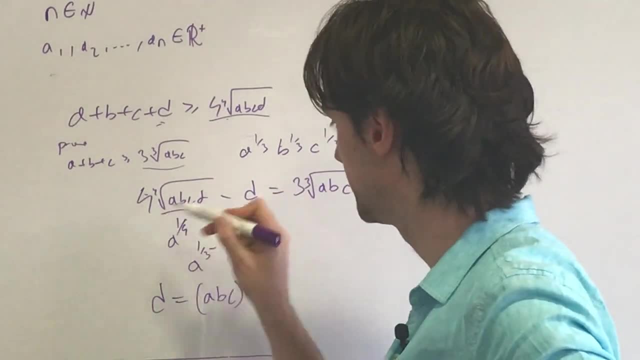 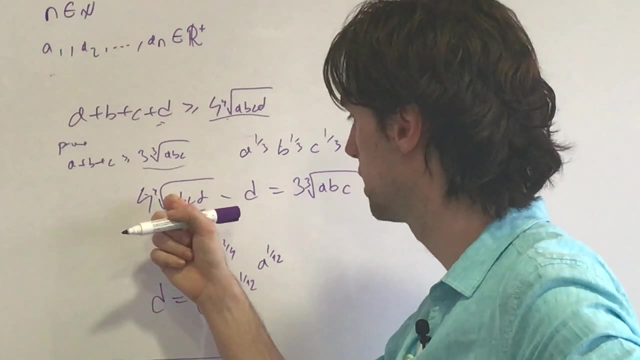 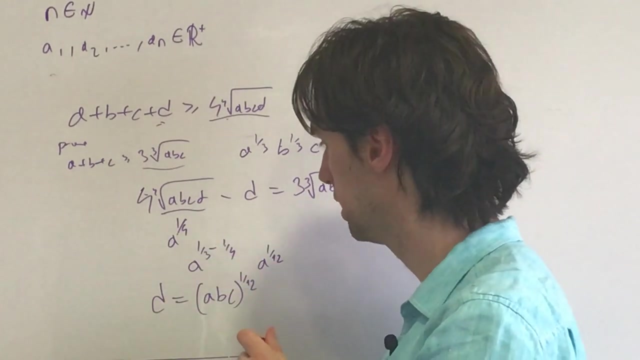 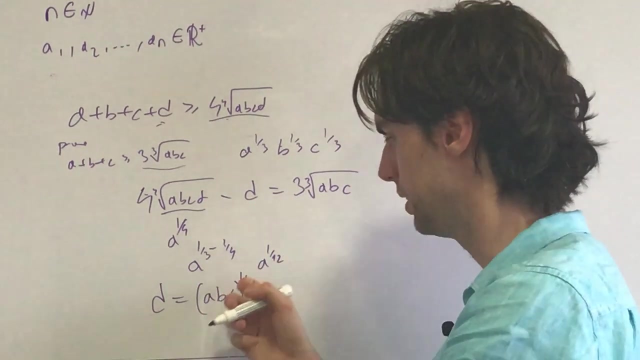 well, we get that. this thing right here transforms into what we get: a to the power of a Third. b to the power of third. c to the power like this all transforms into. Actually, but wait, we have not really that. We have right, it's not- d to the 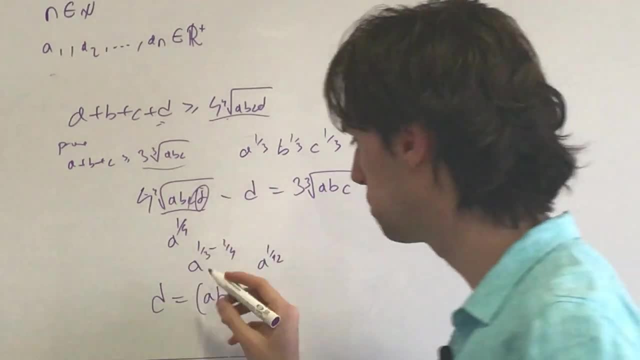 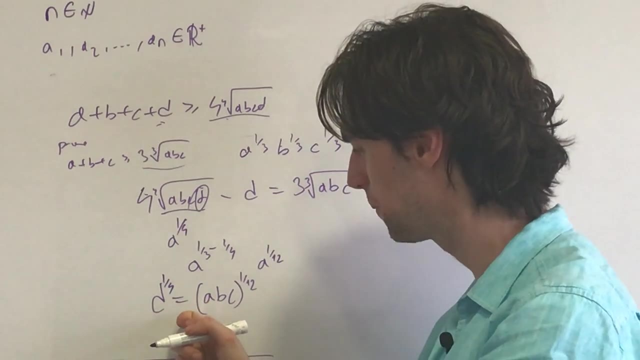 we need to have d right now is d to the power of a fourth. right Actually, d here is d to the power of a fourth. So what we really need is to have d equal to a, b, c to the power of a third. 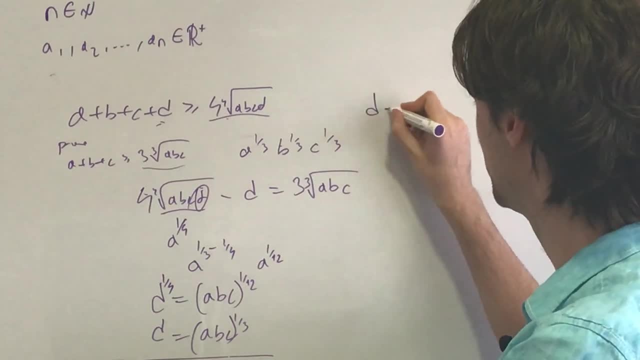 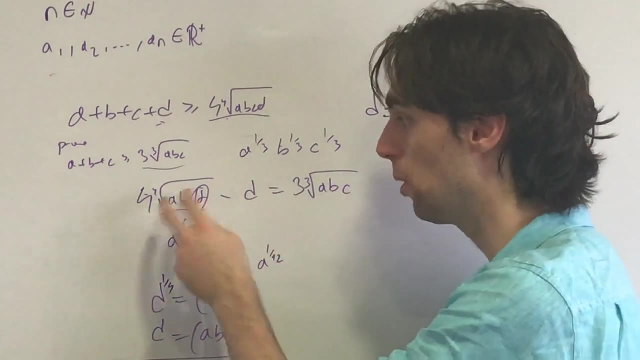 Which then will give us what we need. So if we place, d is equal to the cube root of a, b, c. we'll have here. we'll have that this is equal to four a b c times a to the third, b to the third, c to the third. 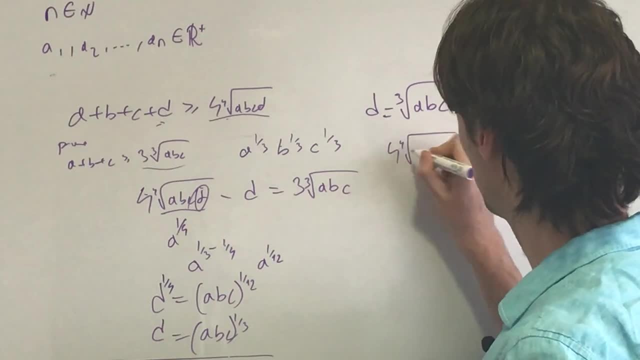 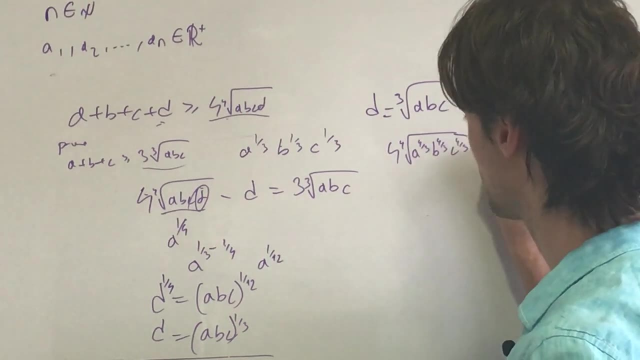 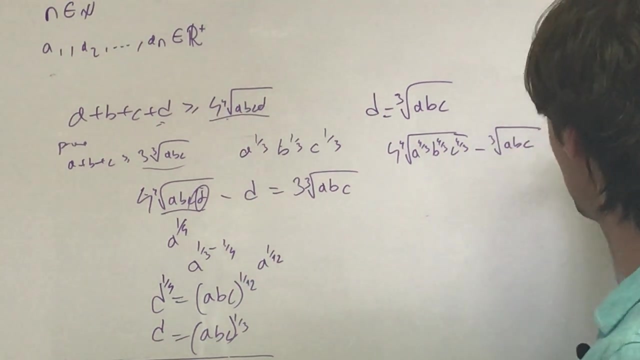 which gives us, so this is going to be four times four, to the a, to the four over three, b to the four over three, c to the four over three, minus the cube root of a, b, c, and this is going to be equal to three times. 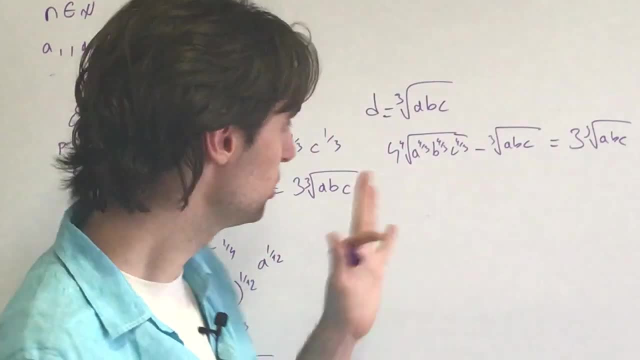 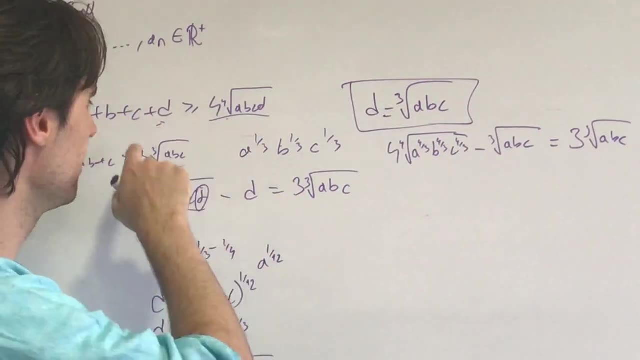 the cube root of a, b, c. So if we put d to be equal to this in the n equals four case, then from here we get this. Now the question for you is- and I invite you to take 20 minutes: 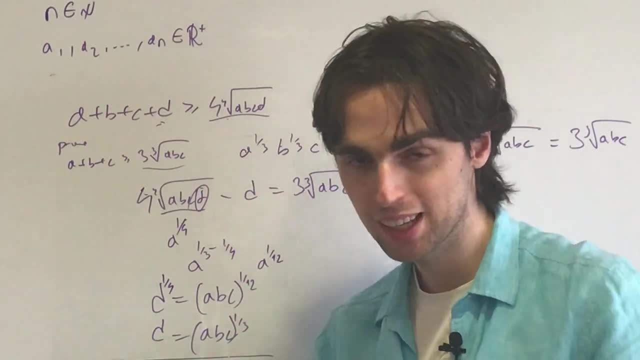 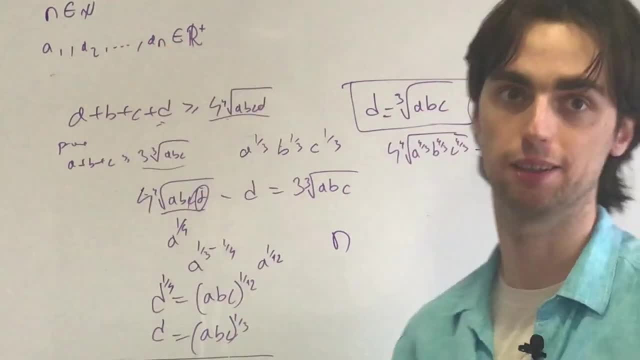 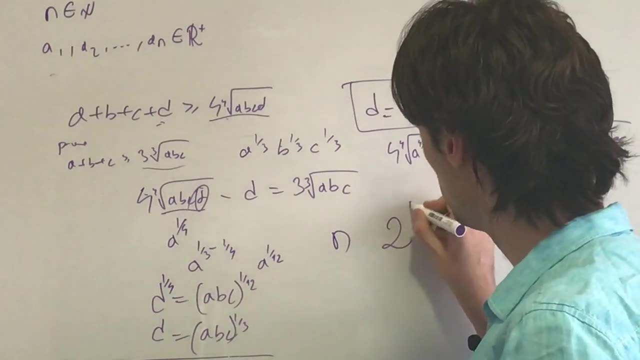 you're proving something for an n right For a one through a n. You want to prove the general a, m, g, m inequality. So prove it for some two to the alpha that's greater than n, And then figure out now if you know that. 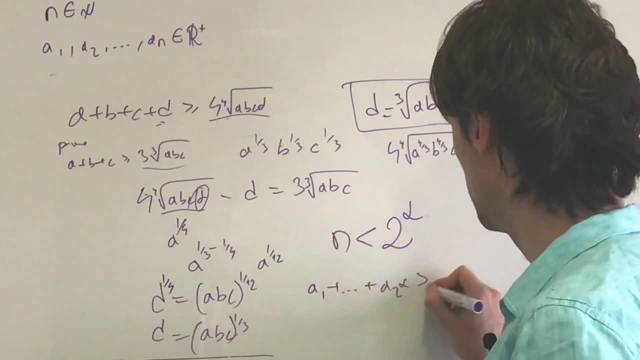 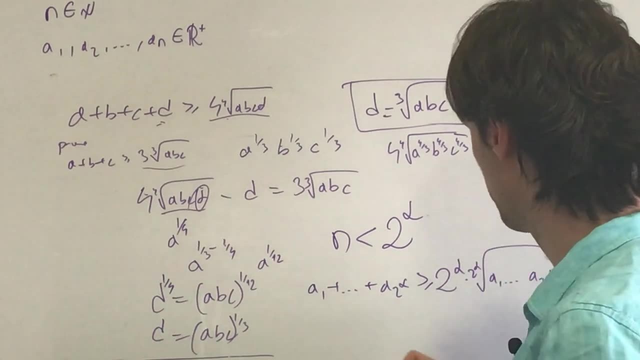 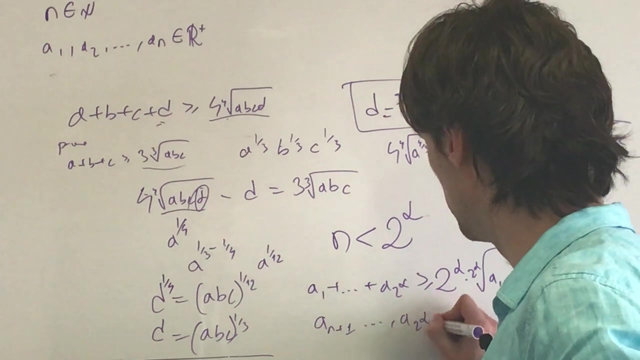 a one plus- hold on wait- a to the two alpha is greater or equal to two to the alpha, times the alpha through of a one through a two to the alpha. Figure out what you need to solve to set a n plus one all the way to a to the two to the alpha. 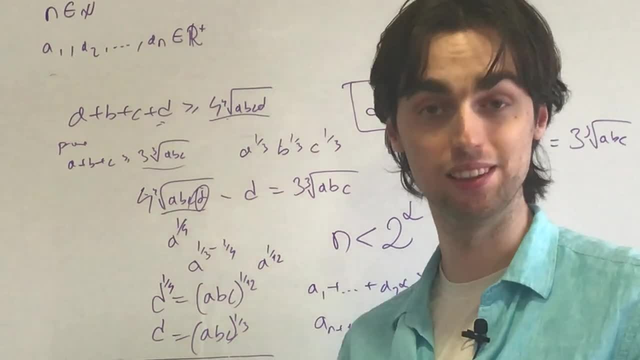 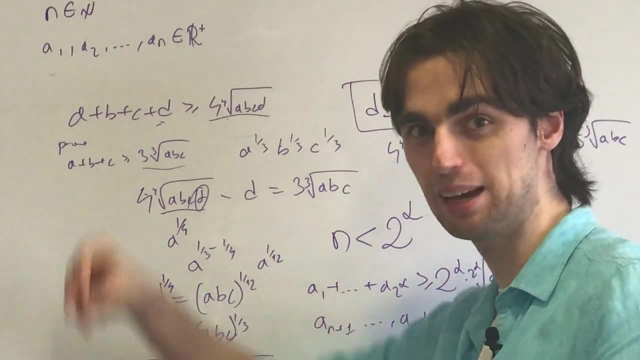 such that you get the inequality that you need. So now, without further ado, I invite you to pause for 20 minutes and try to figure that out. And here's the next step. We have this via induction. we know this is true. 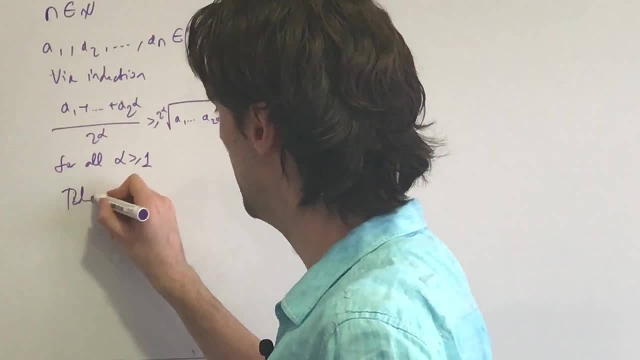 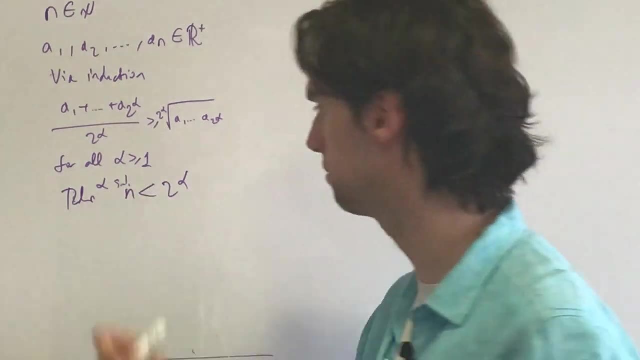 Now we have: take n less than two to the alpha, or take two to the alpha less than n. Take alpha such that two to the alpha is less than n, I mean is greater than n. And now what do we have? 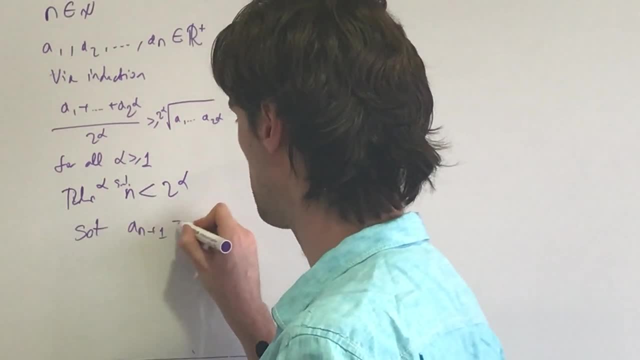 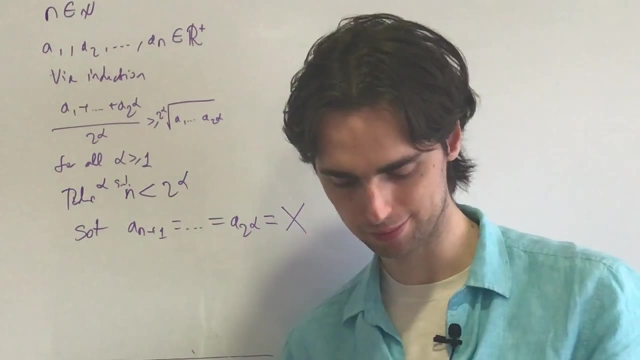 Then we need to set a n plus one is equal to a. two to the alpha is going to be equal to some x, right, We'll figure out later what this x needs to be. Now let's do the calculations. What do we have? 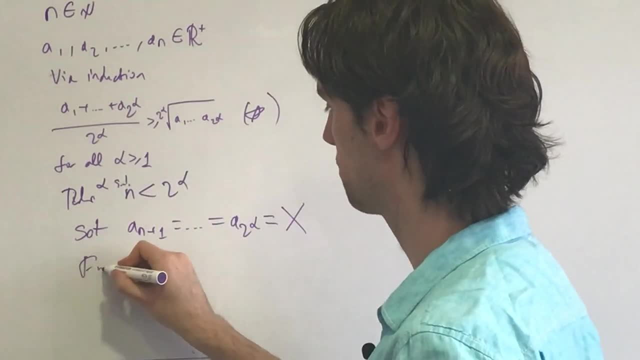 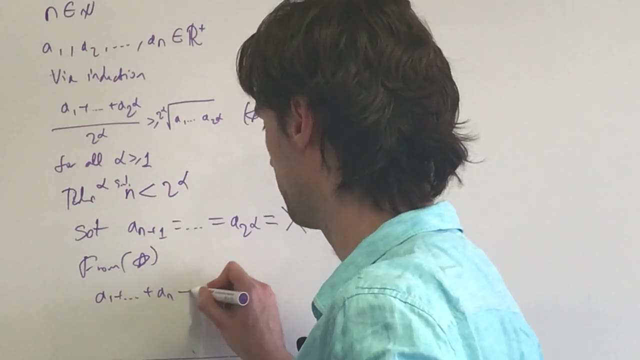 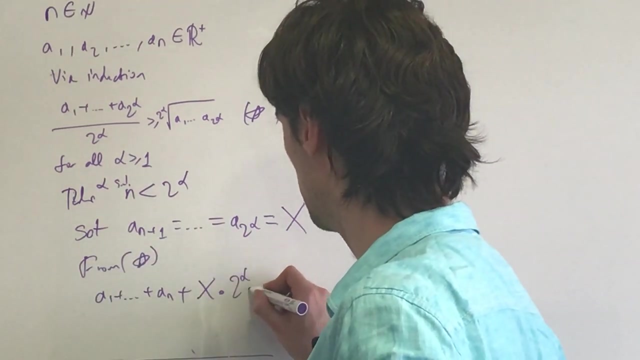 Then from here, let's call this star. So we have from the star. we know that we'll have a one plus a n, plus how many x's. We have x times. what is this? This is two to the alpha minus n. 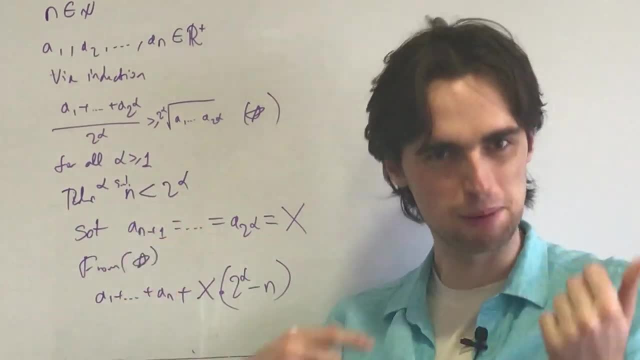 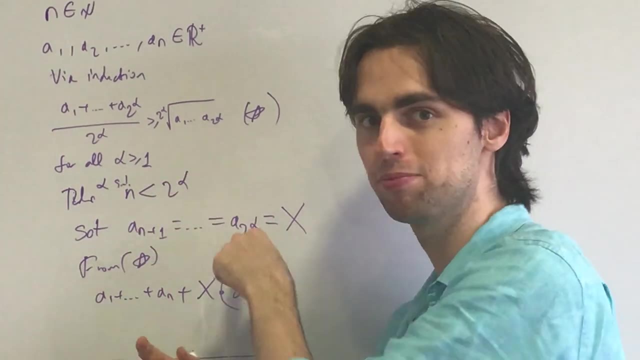 How do I know? there's two to the alpha minus n things Here. this is like a little, just a tip. I sort of saw once and always use is this is n plus one, n plus two to the two to the alpha. 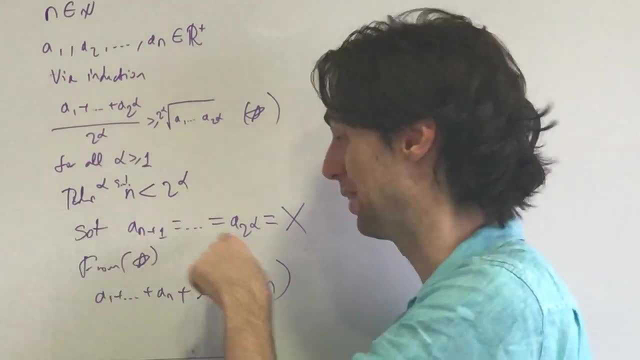 Now, how do I count these? Oh, it's difficult. Well, if I decrease n for every single one of these indices, I'll have a one through two to the alpha, So a to the two to the alpha, like now, it's like one, two, three. 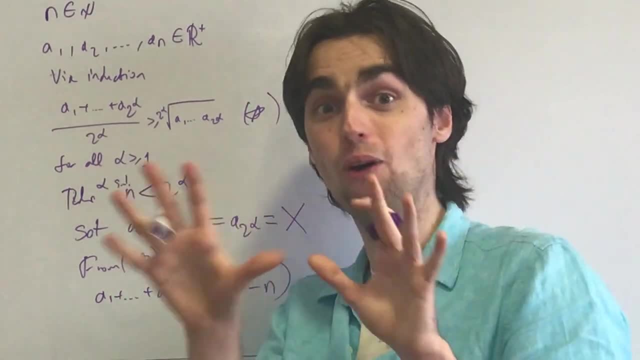 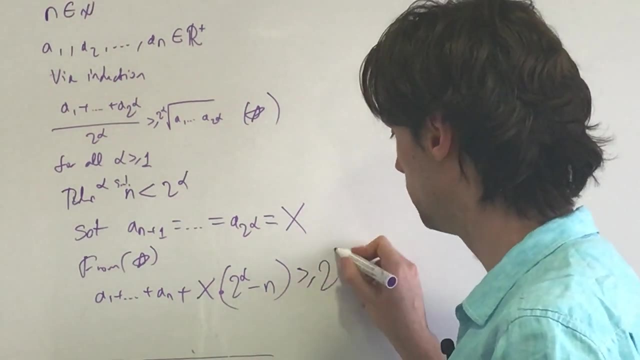 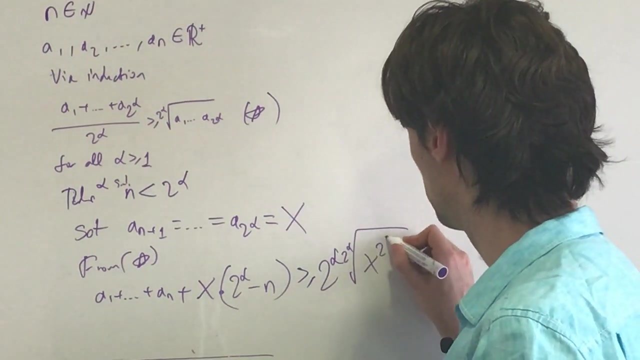 two to the alpha minus n. It's just easier for me to figure out, like oh, how to actually count when I do that. But anyways, back to the problem we have. this is greater or equal to two to the alpha times d, two to the alpha root of x to the power. 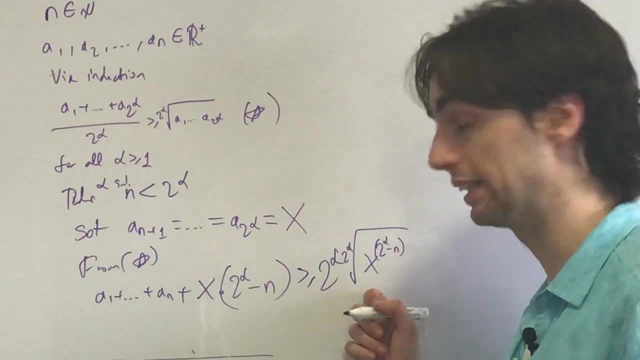 of two to the alpha minus n, because that's how many times we're multiplying this times, all these other ones, a one through a n. So that's how many times we're multiplying this times, all these other ones, a one through a n. 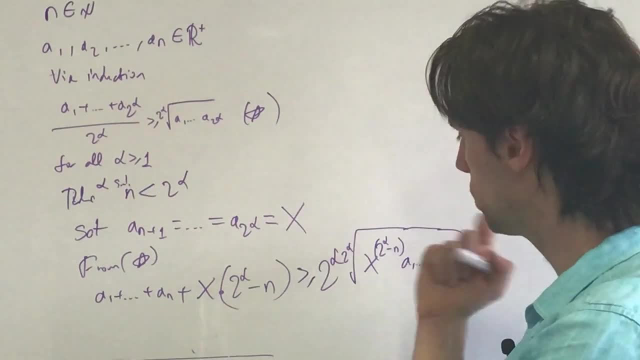 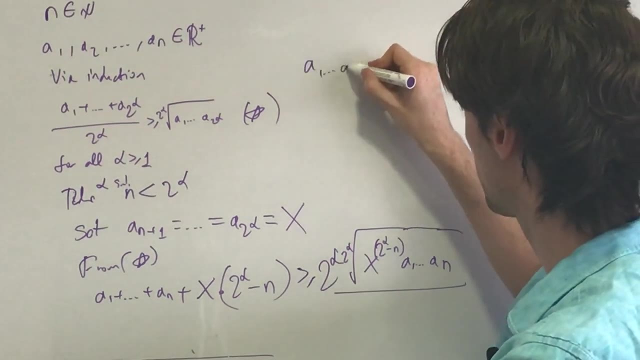 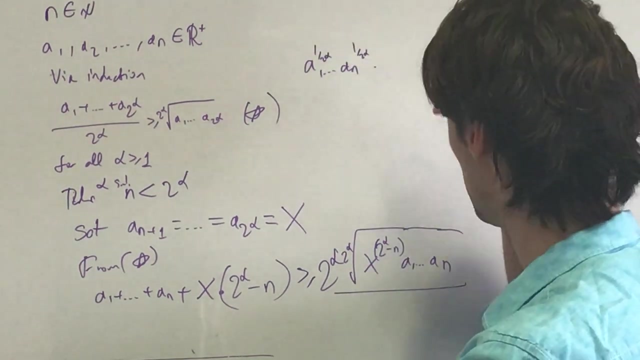 Okay, now let's see. what do we actually need? Well, we need this thing right here. We need a one through a n like this is all to the power of one over two alpha, one over two alpha. We need this times x to the power of two alpha minus n. 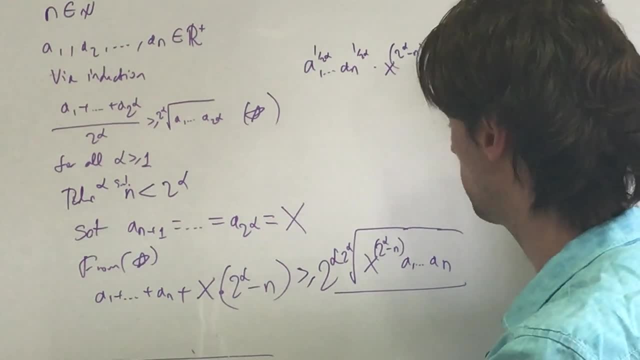 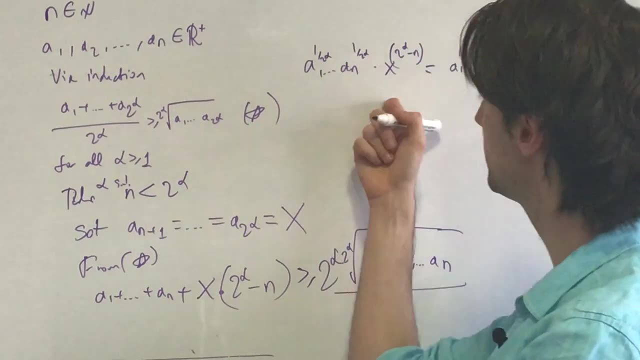 We need this to be equal to a one to the power of one over n, And so on and so forth: a n to the power of one over n. So now, what does x need to have for a one? Well, we need to have: 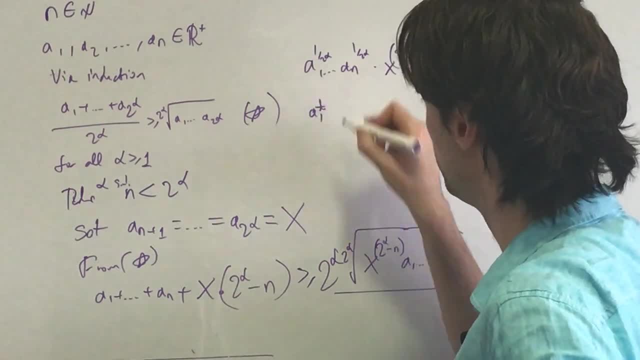 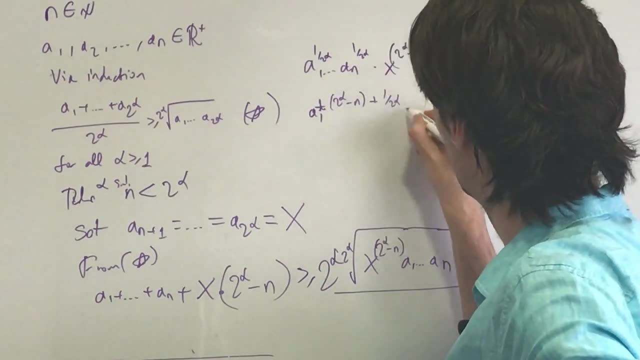 if x is going to have a one to the power of some, say t, then this is going to be to the power of two to the alpha minus n, plus one over two to the alpha, And this needs to be equal to a one to the power. 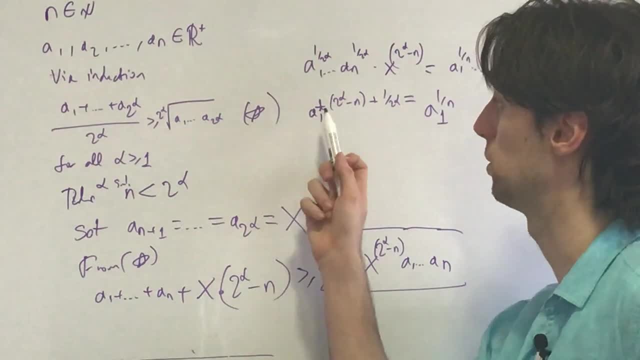 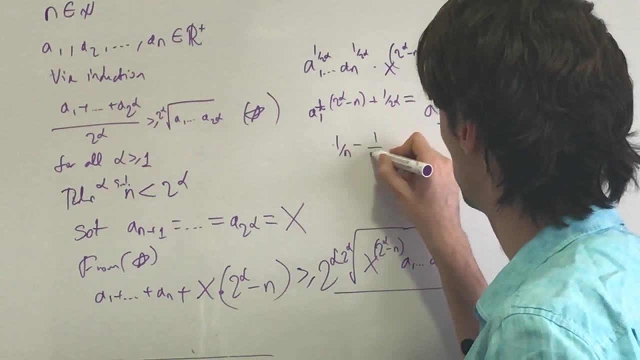 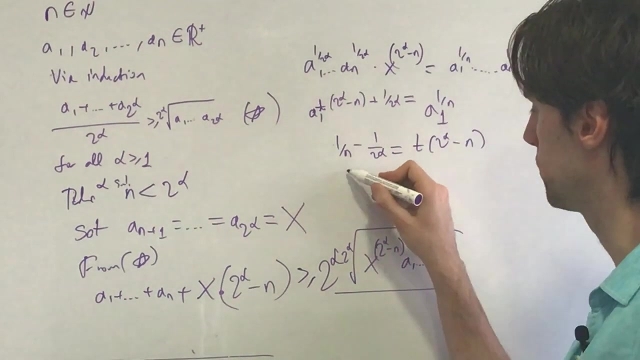 of one over n, right, If it's to the power of some t. And now we solve for t. We have one over n minus one over two to the alpha is equal to t times two to the alpha minus n. And from here what do we get? 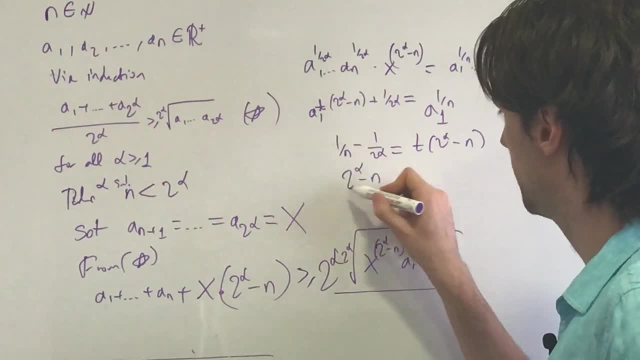 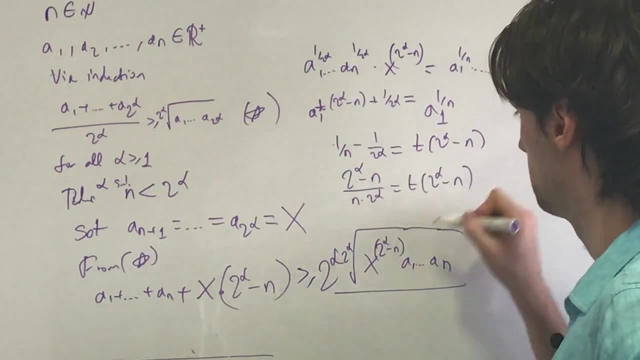 We get that. this is two to the alpha minus n over n times two to the alpha is equal to t times two to the alpha minus n. These two cancel out and you have t is equal to one over n times two to the alpha minus n. 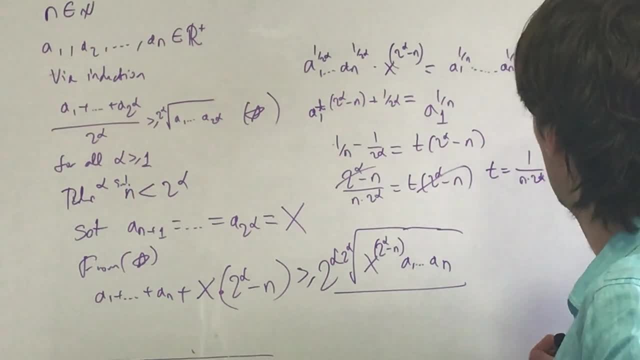 And now we have a t times two to the alpha, minus n times two to the alpha. which means what? Which means that, okay, x. So x is going to be equal to a, one to an, and every single one of these to the power of what? 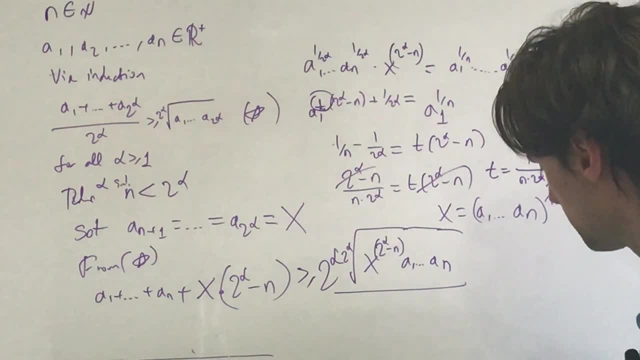 One over n times two to the alpha, And then what will happen here is this is going to be to the power of one, One one. then we're going to have this over n times two to the alpha, plus n times two to the alpha. 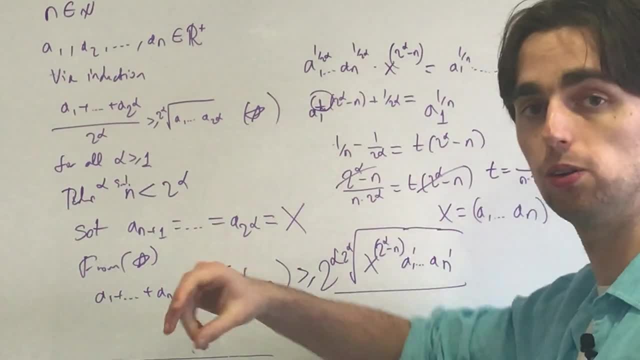 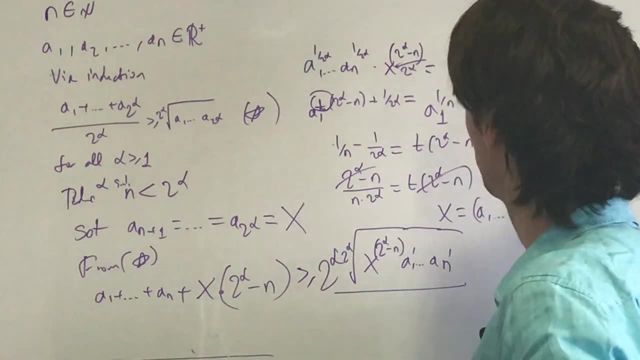 And let's see actually what happens when we do this And if we've made a mistake. so next step is- and actually we have made a mistake. I just saw I forgot to divide this by two. to the alpha Right, So I forgot to divide this. 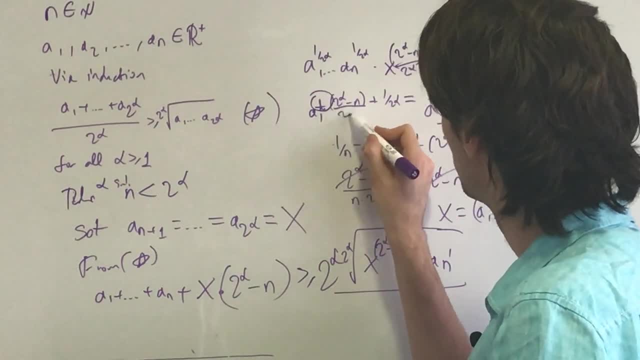 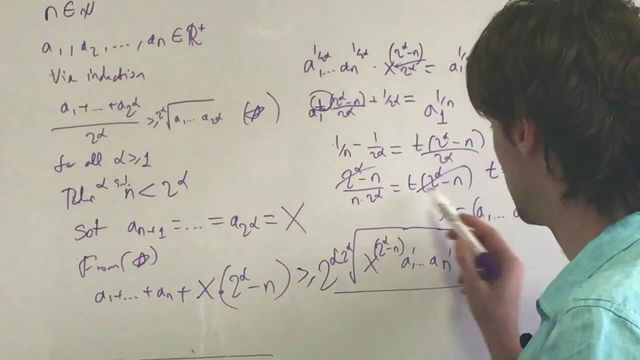 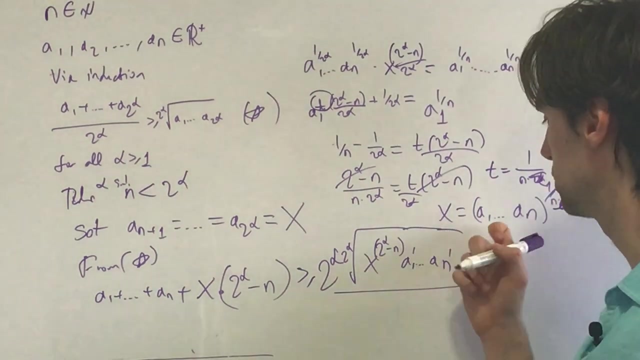 Now we have. this is also over two to the alpha, which changes the calculations, but it only changes them a little bit. over two to the alpha, which means t doesn't have a over two. So this over two to the alpha t is equal to one over n. 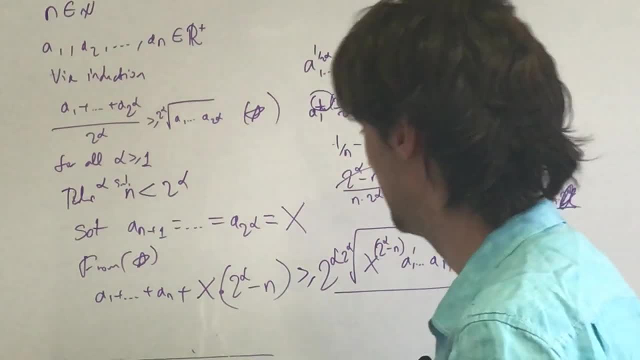 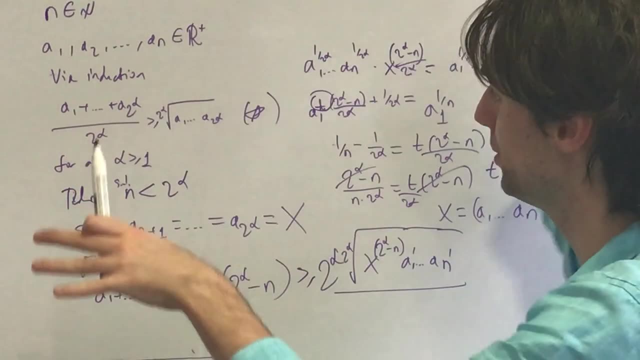 So x needs to be a one times a two the way till an times one over n. add to the power of one over n And what happens when you plug this in and do the math is you get is that a one times a, two times an times. this. 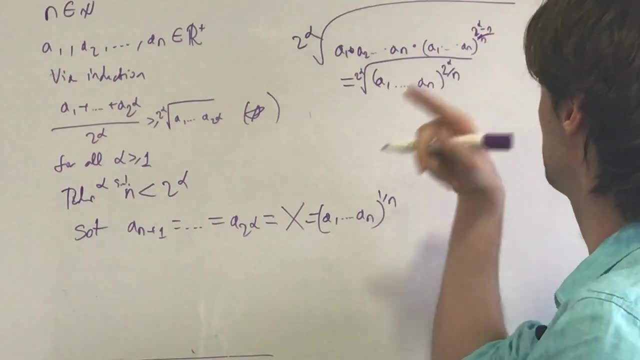 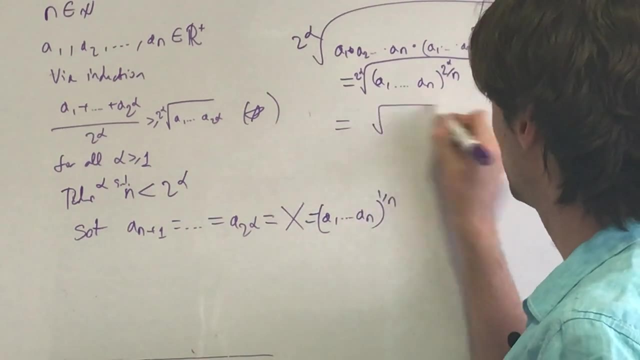 to the power over n times. How many times we have a two to the alpha minus n, We get that the right-hand side of the inequality turns into this is going to be equal to a one times a n- The two to the alpha, and this cancel out. 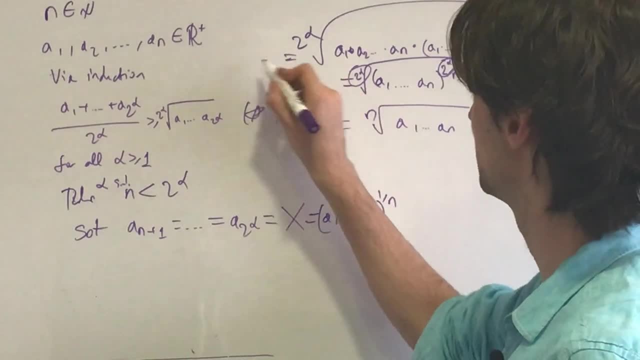 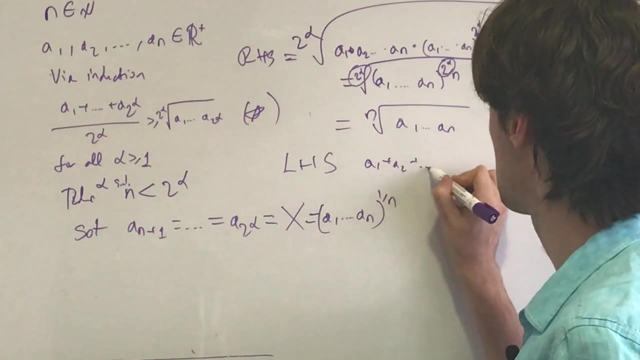 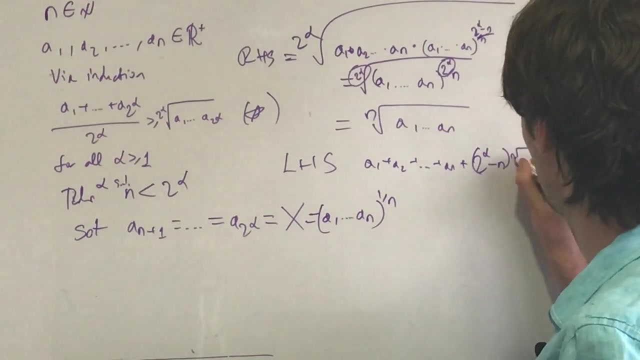 and we're left with one over n. So that goes in here. So this is what the right-hand side is equal to And the left-hand side a one plus a two plus a n, plus two to the alpha minus n. So this is going to be equal to a one plus a two plus a n. 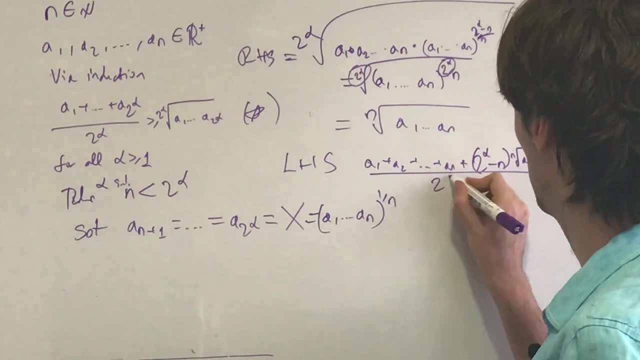 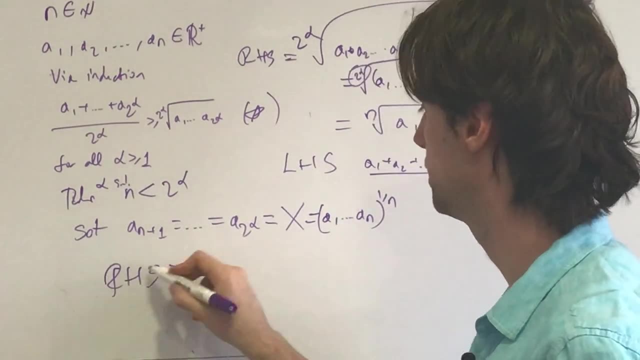 times the nth root of a, one through a n, all the thing over two to the power of alpha. Now, when you do, right-hand side is greater than or equal to is less than or equal to the left-hand side. When you multiply everything through by two to the alpha. 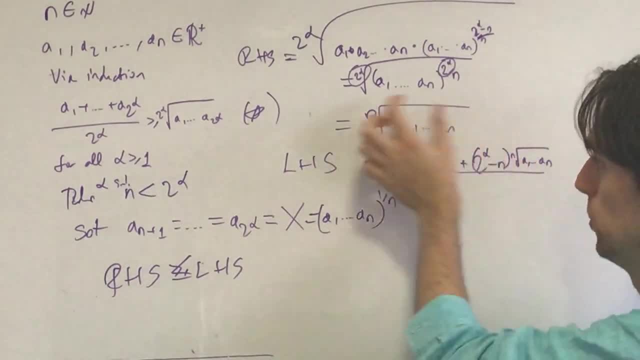 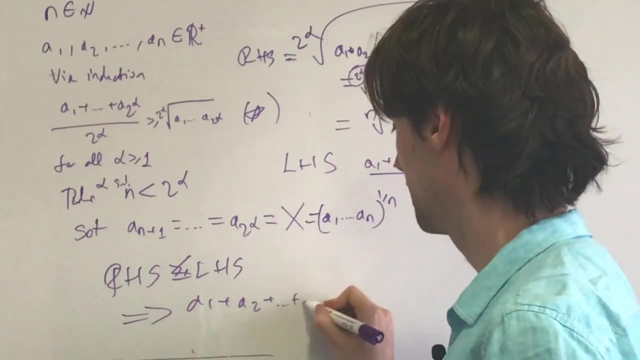 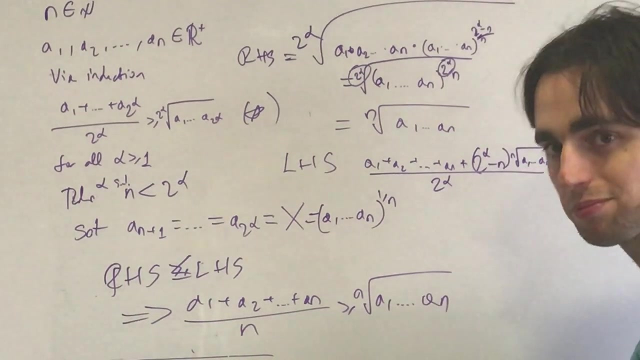 these things, then this cancels, this thing cancels out with this and of them remain, And then this implies that a one plus a two plus a n over n is greater than or equal to the nth root of a one through a n. 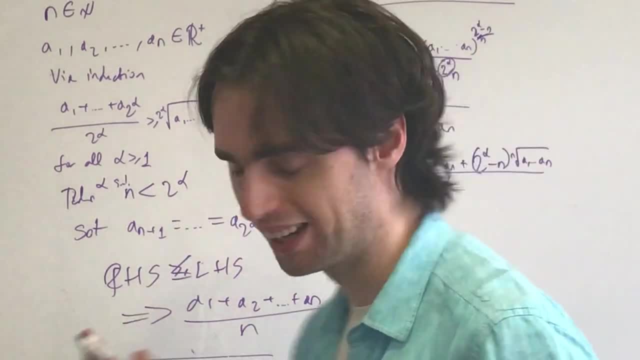 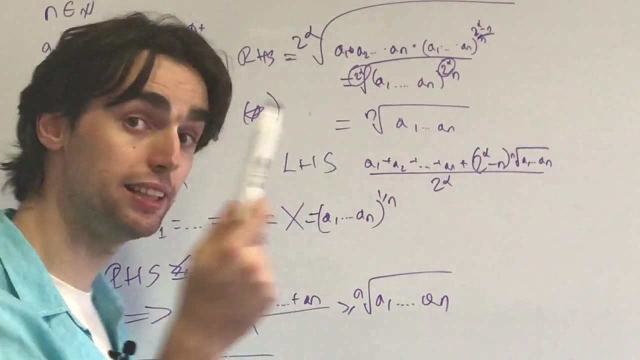 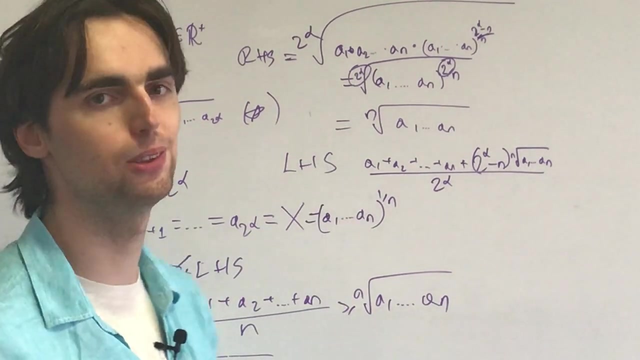 And this solves the arithmetic a m g m. This proves the a m g m inequality And we have the equality needs to hold true where it holds true for the inductive case. So when a one is equal to a, two is equal to a three. 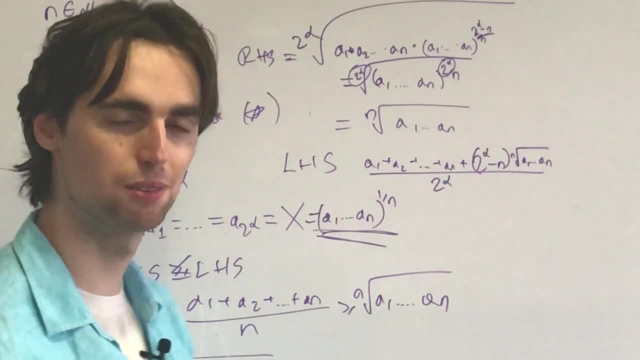 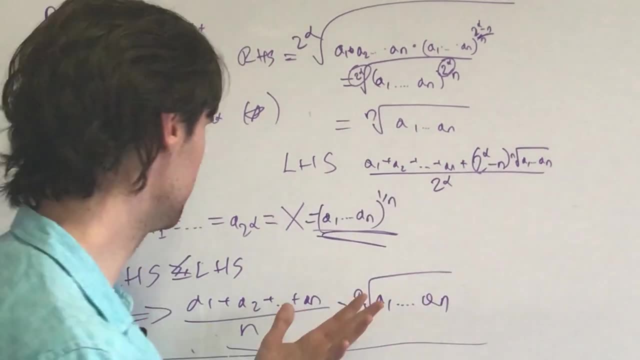 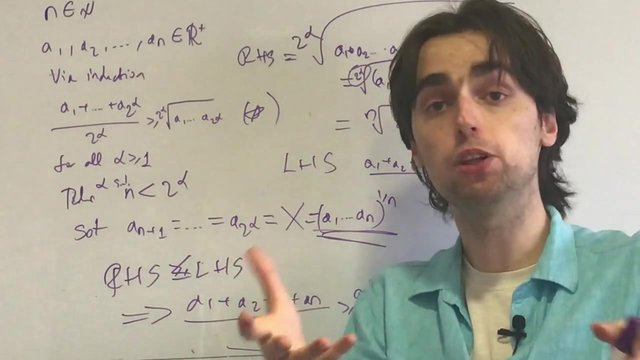 is equal to a, n is equal to this For all these AIs. and now this solves our. this proves the a, m, g, m inequality. And now you know like. what I like about this proof is it taught me a new concept. 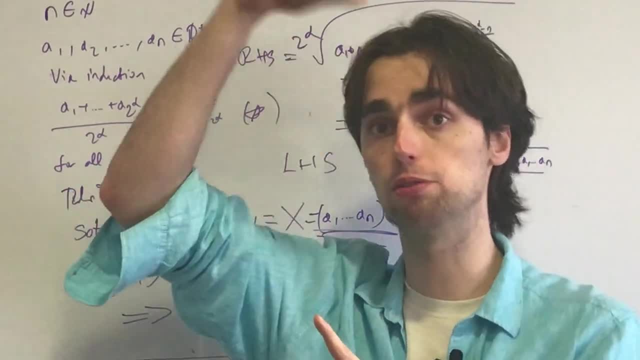 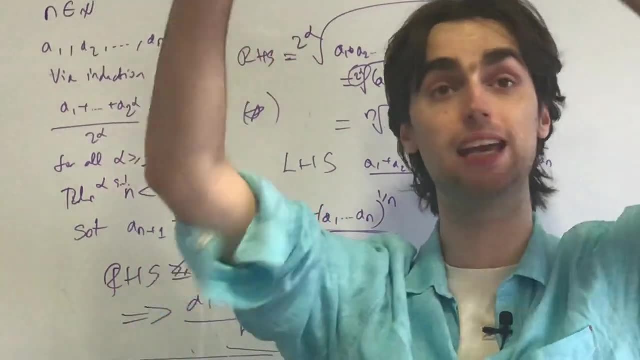 It taught me a new concept of like going inductively to the power of two and then figuring out. wait, I can go to inductively to something, have a proof for some big M and then use that fact to figure out smaller cases. 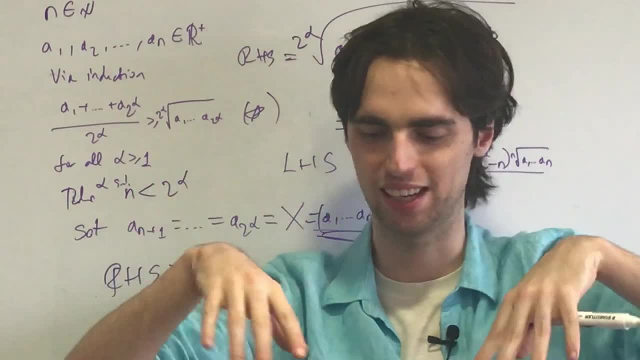 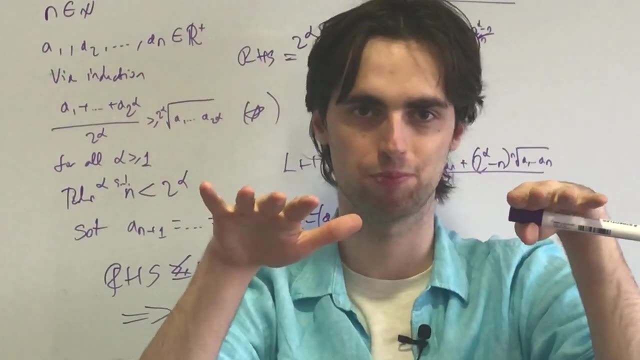 Like I don't need. I can go inductively back and forth Like: okay, I have one, I have two, three, I don't have it, let me go to four. I have four. now I have three. 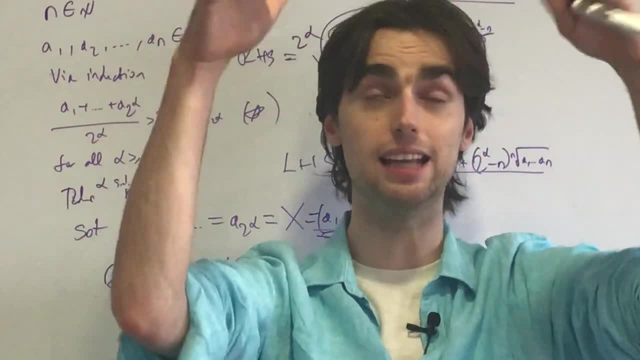 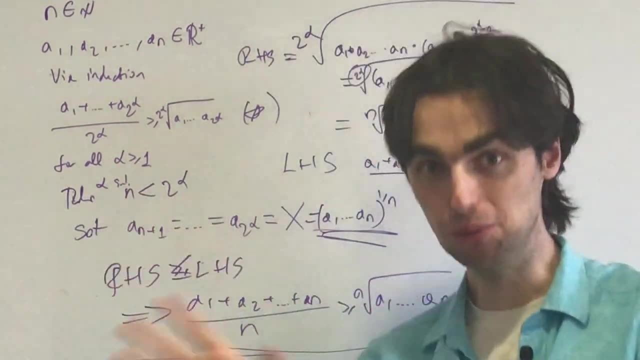 And I have. okay, I don't have five, six, no Eight, I have eight. Okay, now I have five, six and seven, And I think this is like a really cool way to think about how to prove something in general. 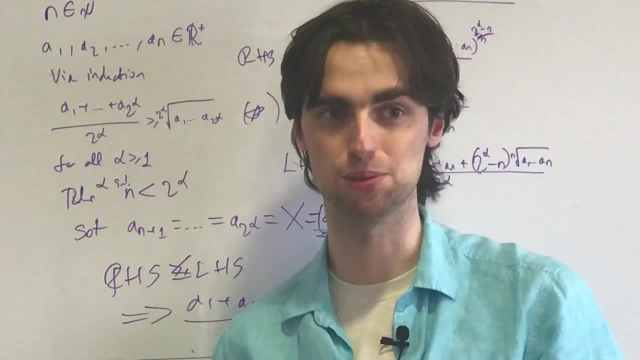 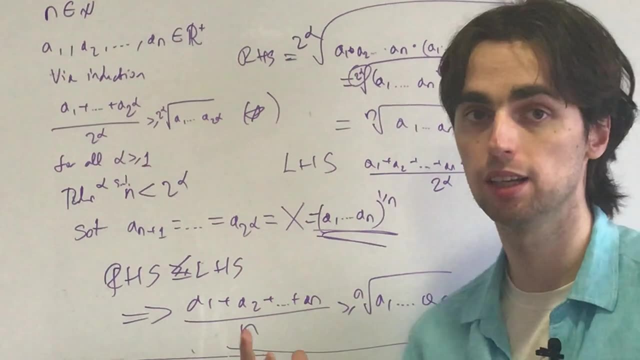 And it also got me an intuition for how this inequality can be proved And why it's also difficult if you don't know it. like for some odd numbers event, it's very hard to use something else, because it's like this is the proof. 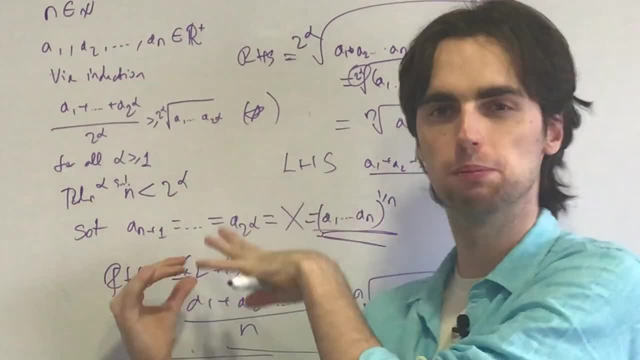 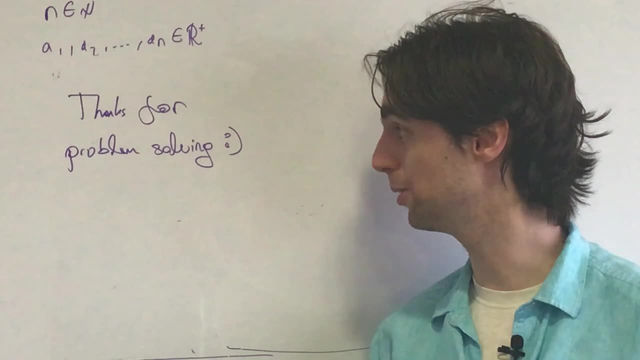 and you know what the proof is and you know that you can't really get to it by other ways. So this finishes up our AMGM inequality And, as always, thanks for problem solving.